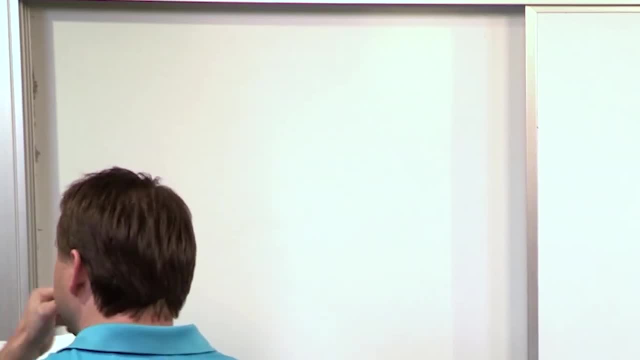 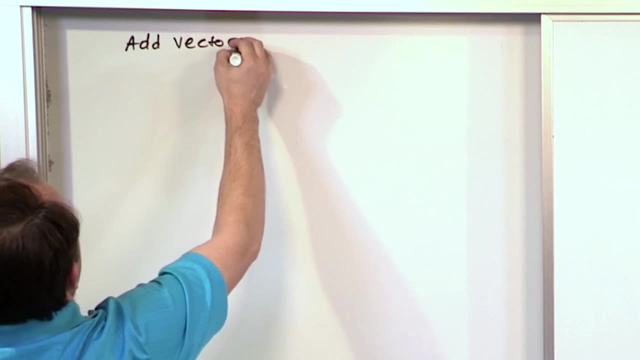 like that, But again, we will review it, as we always have. So when you add vectors, you can do it one of two ways. So add vectors. The first way is graphically, And usually this is what people are taught early on, And then, after you get that out of your system, you start to use numbers to. 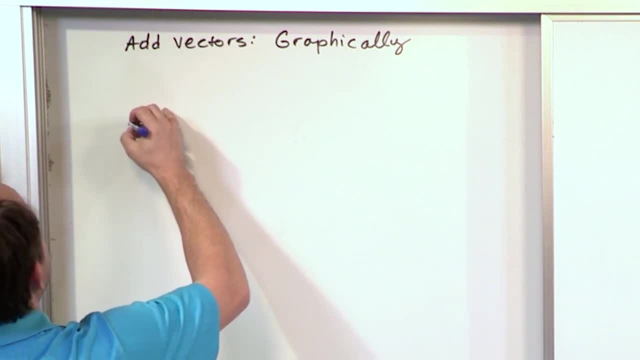 represent everything. But for now we're just going to review real quick. So if we have two vectors, let's say I have a vector pointed this way and I'm calling it a triangle, Vector A, And I have a vector this way, I'm calling that guy vector B. And I wish to add: 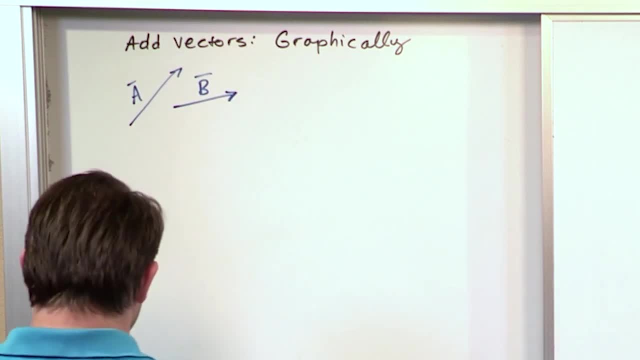 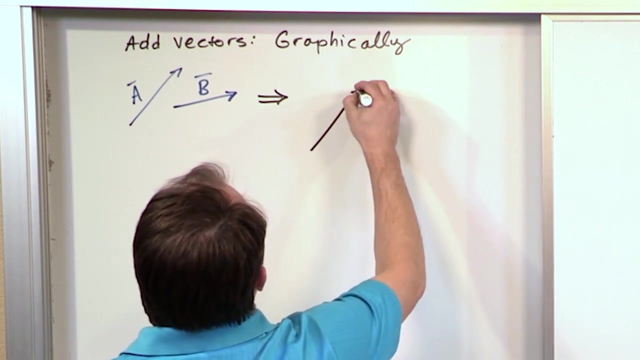 these two vectors together. What you need to do is redraw the situation. So I'll put an arrow here saying that I'm moving from this representation to something else I'm going to draw. And what I'm going to do is I'm going to redraw vector A exactly as it sits, Or pretty close, Maybe, that's. 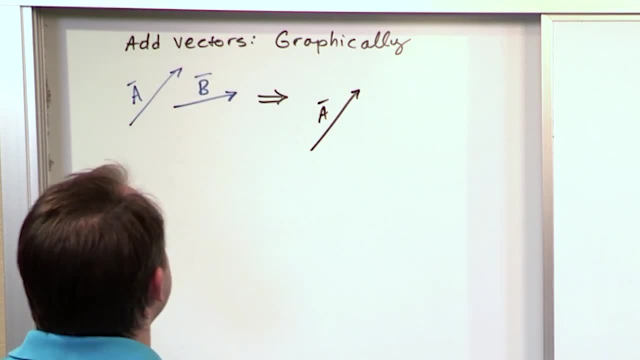 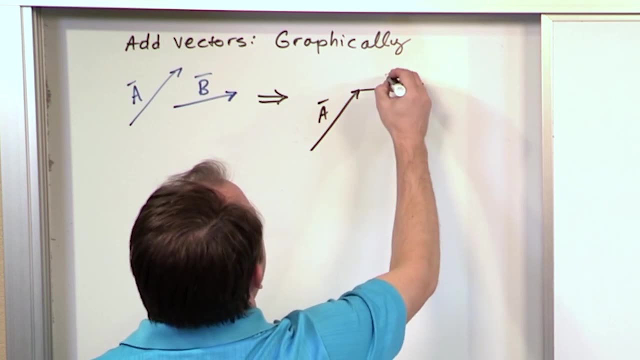 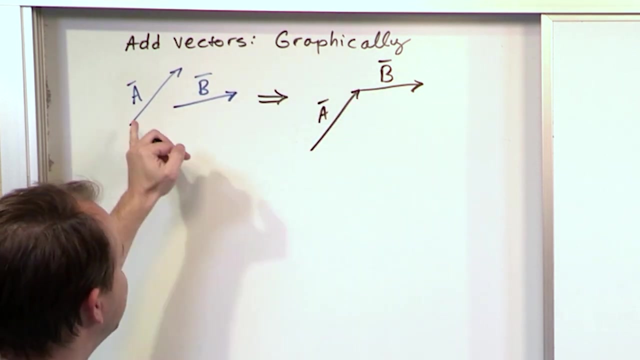 a little bit steeper, But it's attempting to draw vector A exactly as it sits. Vector B- I'm going to draw it head to tail, So this is what we call vector B. So here vector A has the same length and it's pointed in the same direction as what we have here. Vector B has the same length as what we. 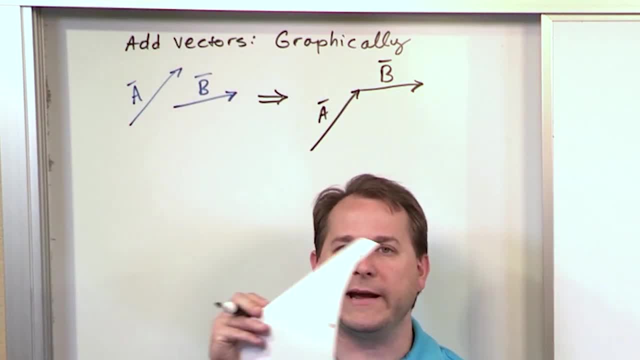 had drawn there And it's also pointed in the same direction. All we did was rearrange how we're drawing it so that we draw it head to tail, Head of this vector to tail of the other vector. And when you have it drawn like that, then you can directly draw. 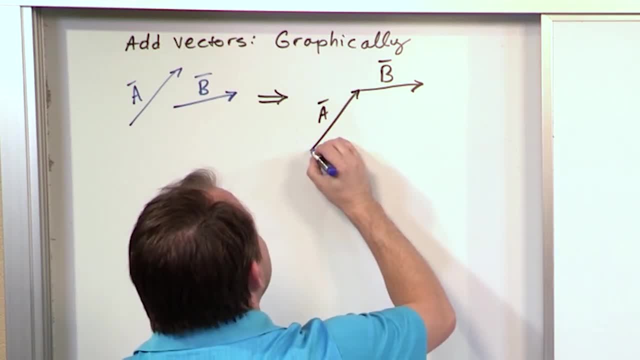 the resultant. That's what we call it. when we add two vectors together. We go the tail of this vector up to this guy right here, And I drew a curved vector. That's never good, So we'll do a little bit better job. hopefully That's a little bit better, And we'll call this guy the resultant. 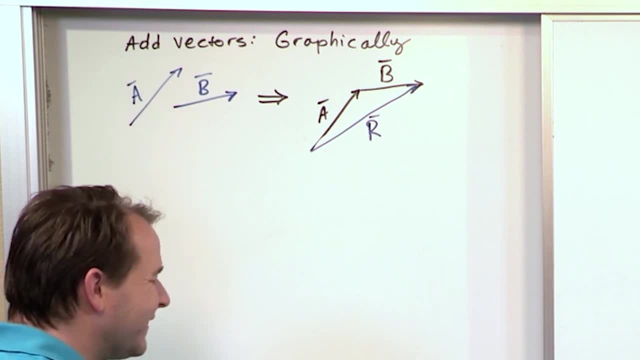 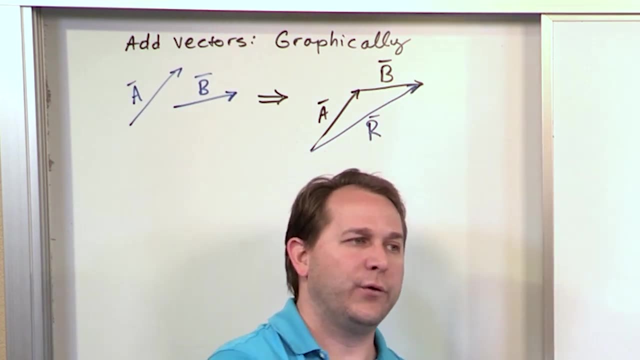 Which is basically the vector that you get when you add A plus B, Because clearly you can't just add the magnitudes of the vectors together. If I have a force here that's 10 newtons and a force here that's 15 newtons, I can't add them together and get something. 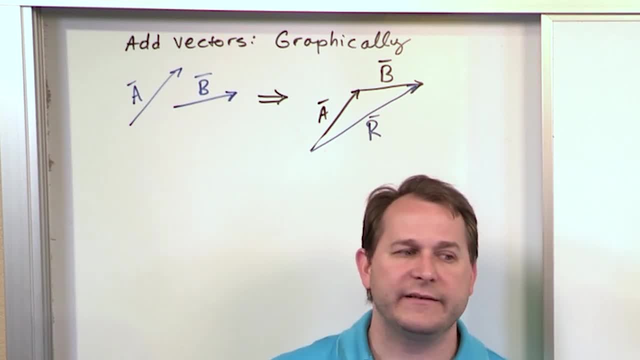 number, Just to just say. well, the resultant is 25 or something, Because clearly they're pointing in different directions. So some of this guy's pulling away, Some of this guy's pulling away, What is the actual resultant is going to take into account the magnitude of the vectors. 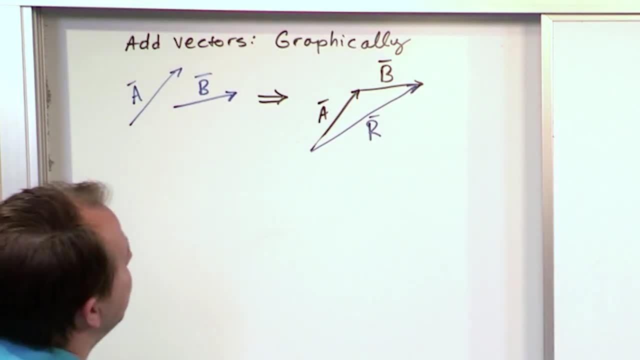 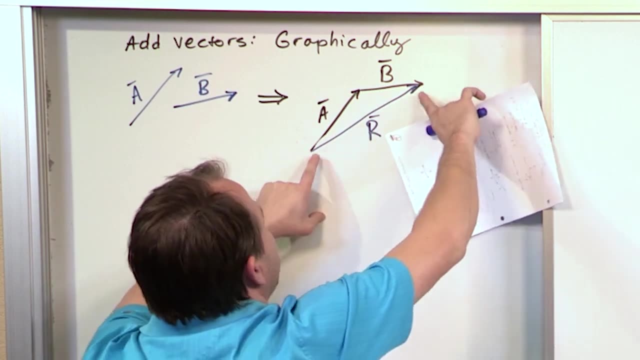 But it's also going to take into account the direction. So the length of A is this, The length of B is this, And the length of the resultant is clearly drawn on the board with the length of that arrow And its direction as well. All right, And so that's the power of the graphical method. It allows you. 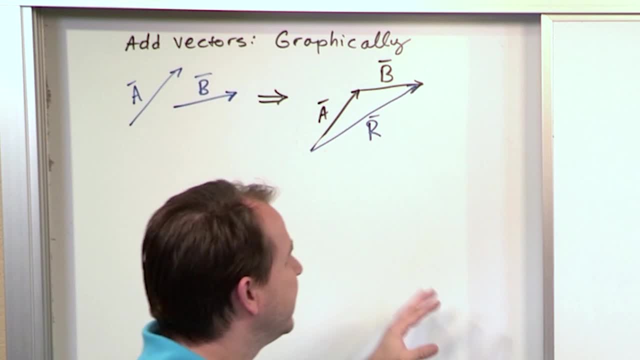 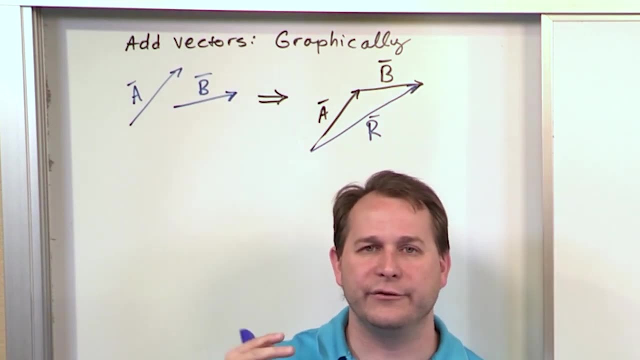 To visualize what you're doing. Unfortunately, this becomes very cumbersome to solve real problems, Because who wants to draw arrows? And besides, this is easy because it's x- y. You know two components, x and y, for the vectors. What if I have a vector with three? 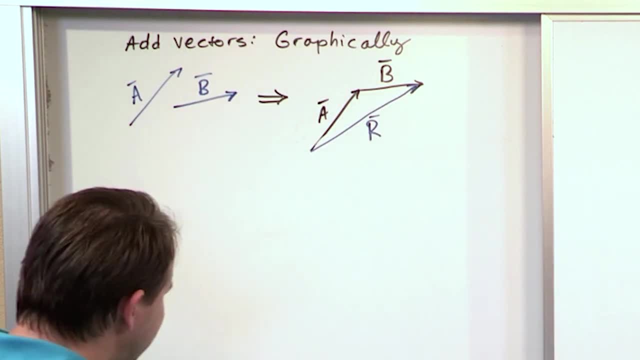 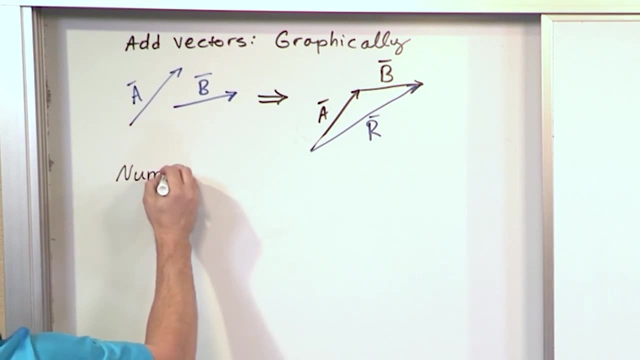 components or more. Very hard to draw that. So we can also add vectors. We did it graphically here, We can do it numerically. We can do it numerically, all right. So to give an example example of that, let me switch back to my blue, And if I have a vector, I'll represent it here. 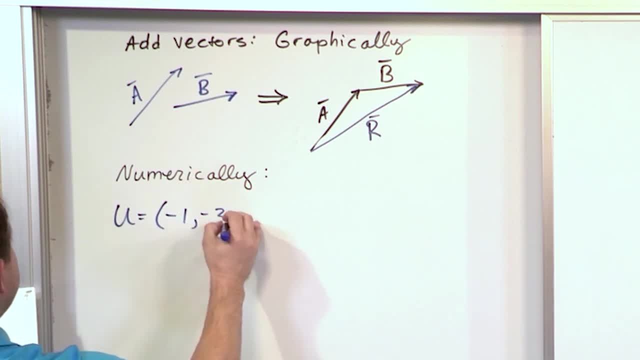 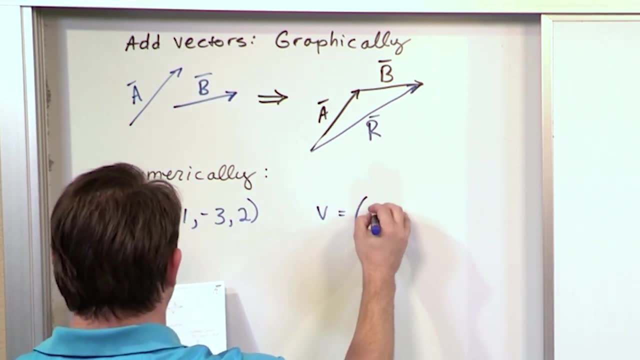 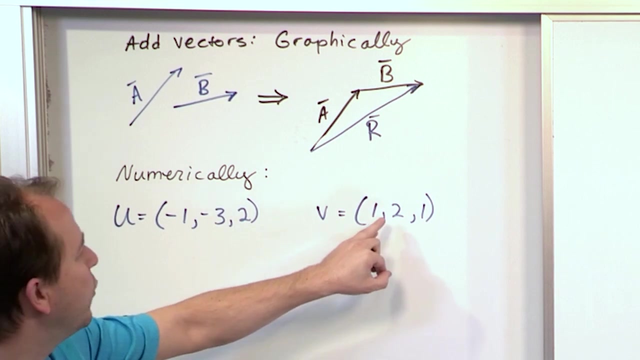 as these numbers negative, one, negative three and two in this, parentheses here- right, That's vector u. Let's say I have another, vector v, which is one, two and one. See, this is a great example. This is a vector with three components: x, y and z, x, y and z. So if I wanted to do the graphical, 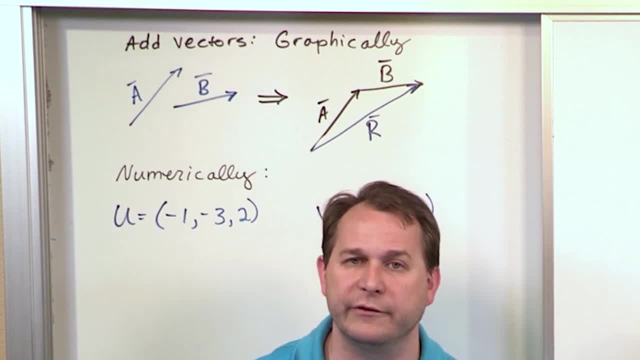 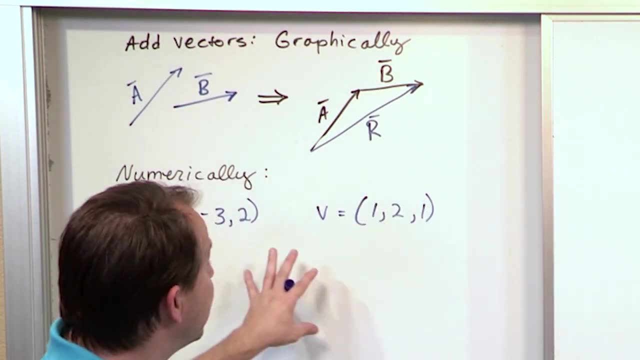 method. I would have to draw it or somehow construct it in three dimensions, draw the other one in three dimensions and then measure the result. and it is real cumbersome in higher dimensions. So we don't really want to draw things for complicated vectors like this. So and also 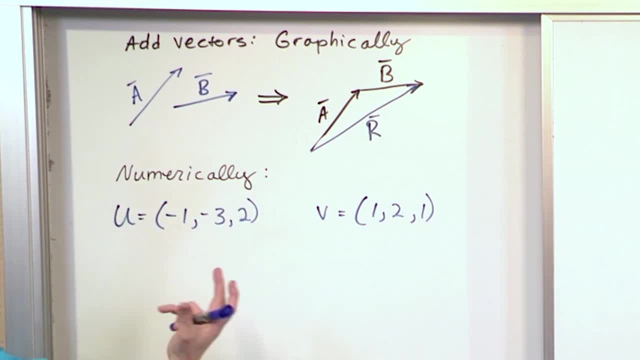 keep in mind. I'm writing them as numbers with commas, but you already know by now that you can also represent it as a column matrix: negative, three negative, one negative, three positive, two, and this one will be one, two and one. We can represent it as a column matrix, I'm just choosing. 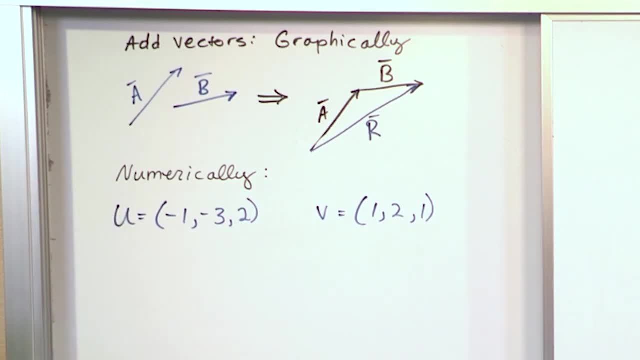 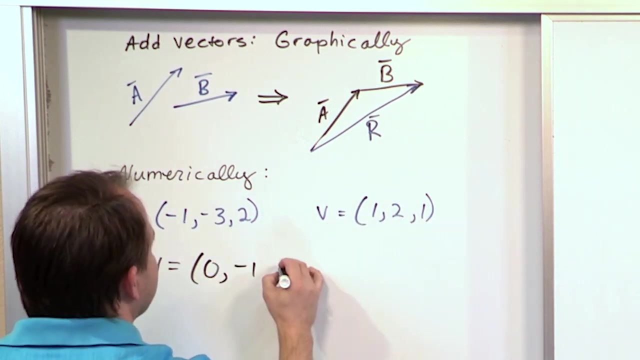 this representation now. But to add them we can say simply: u plus v is equal to. we add the x components together, negative one plus one is going to give me zero. We add the y components together, giving us negative one. We add the z components together, giving us three. So you see, we just simply add. 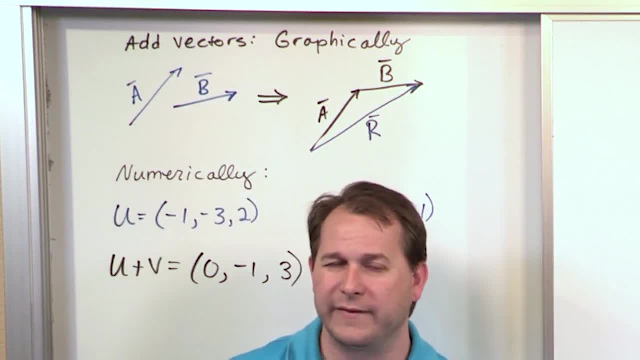 everything together and notice that I told you before that a vector is really represented in linear algebra like any other matrix. There's no real difference. Remember, And I also taught you early on how do you add matrices together. You have matrix A and 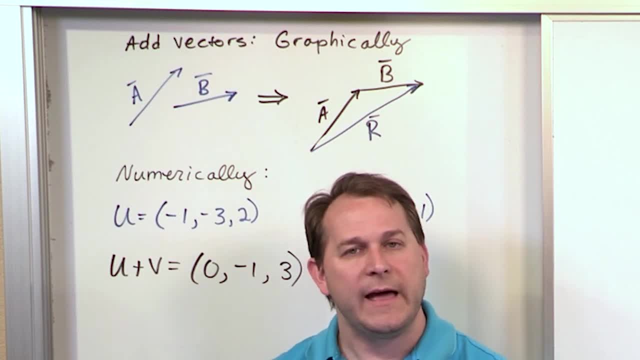 matrix B. The only way you can add them is if they're the same size, and then you add element by element, adding the corresponding elements. So if you think of this as a matrix, it has three elements. If you want to represent it as a column matrix, that'd be fine. That'd be a three by one. 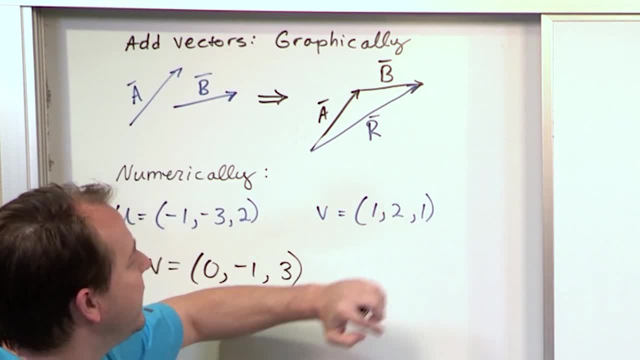 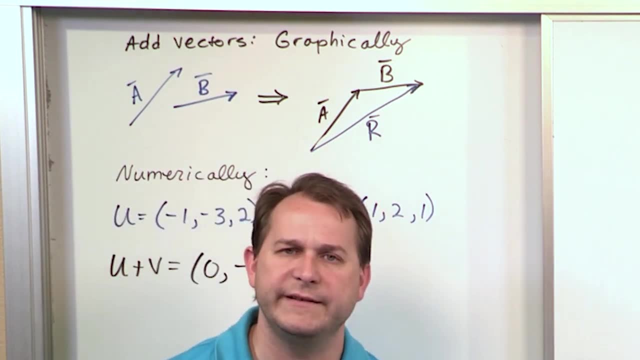 matrix. You also have the same dimensionality here. You have three elements. So we add the first elements together, We add the second elements together, We add the third elements together. So we're being consistent. We're adding these vectors the same way that you add matrices. 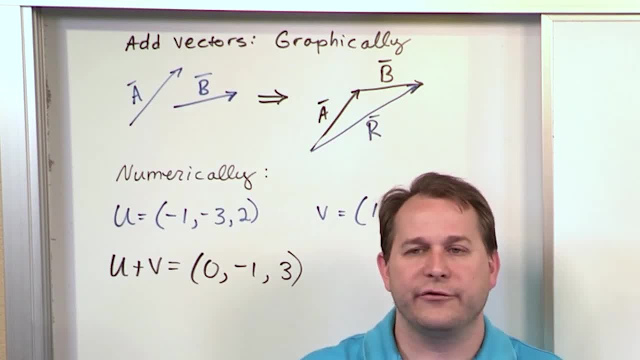 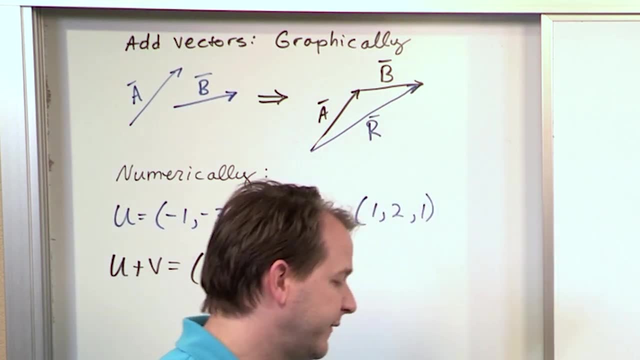 together, And that's again just further proof that vectors really can be represented just like a matrix, because the same mathematical operations that we use on matrices can be applied to vectors. I think it's the same thing essentially. All right, And now what we want to do, now that we've 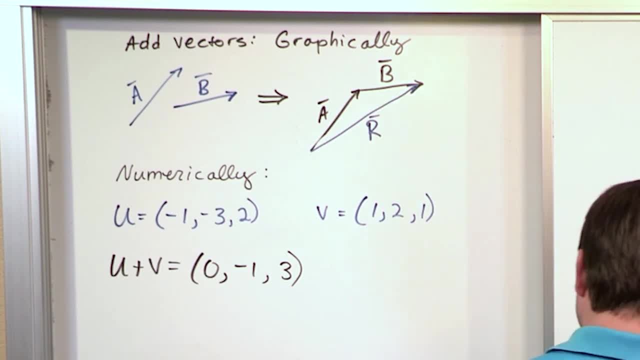 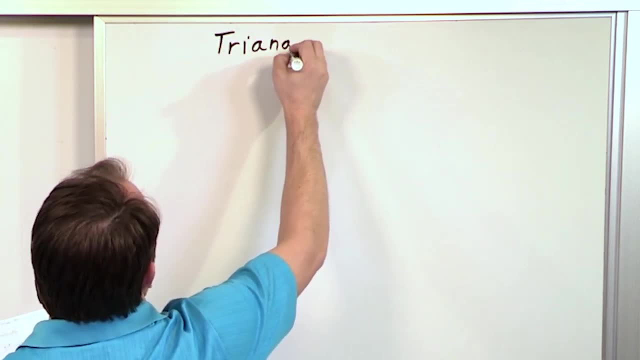 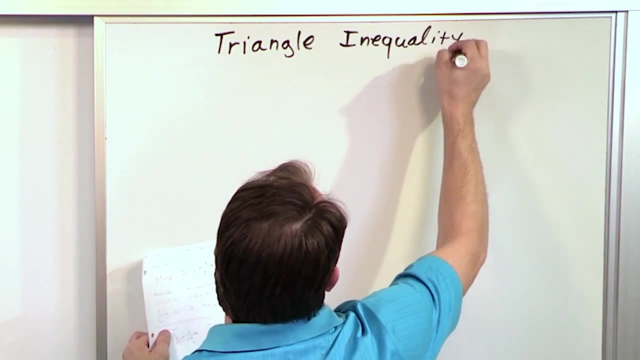 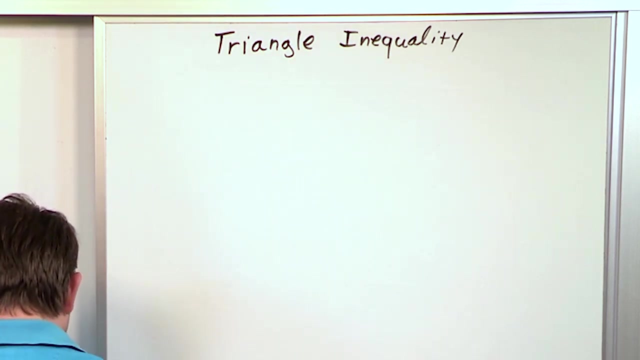 kind of reviewed that basically wanted to review how to add vectors for you. there is. I want to talk about the triangle inequality, The triangle inequality, And in order to do that, you know, what I'm going to do is redraw a picture that I have on the board here. We said, okay, here's vector. 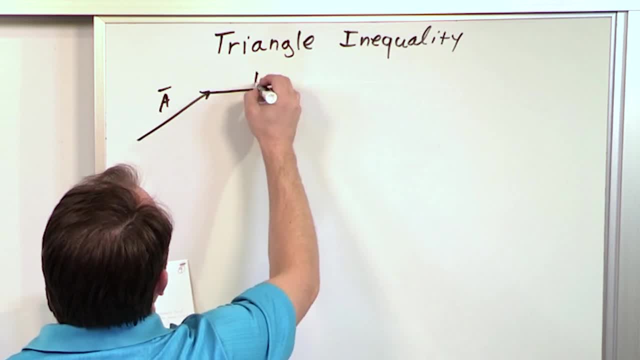 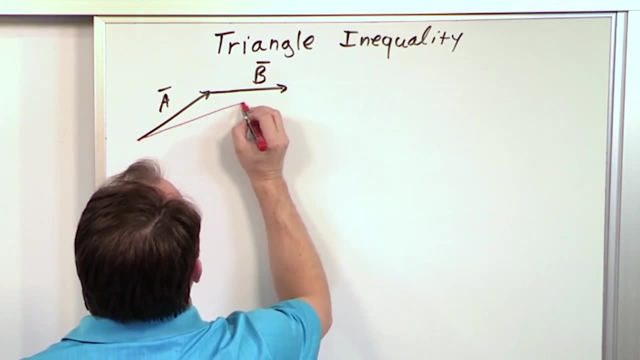 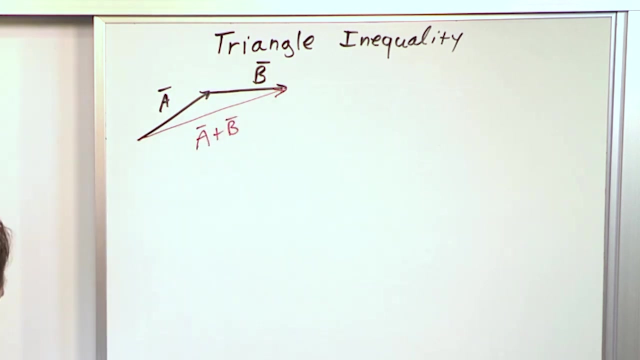 A, and here's vector B And the sum of those when you add them vectorially as you go from the tail of B and we call this resultant, or you could just label it A plus B. Okay, Now the triangle. 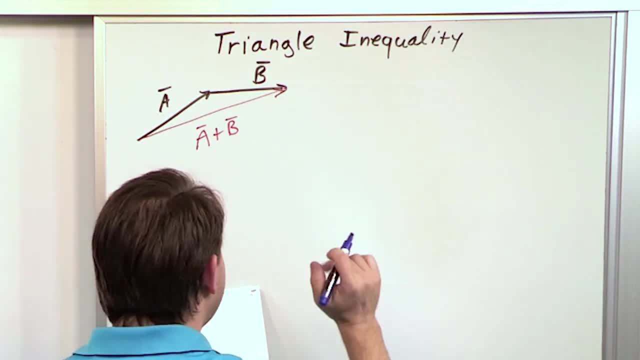 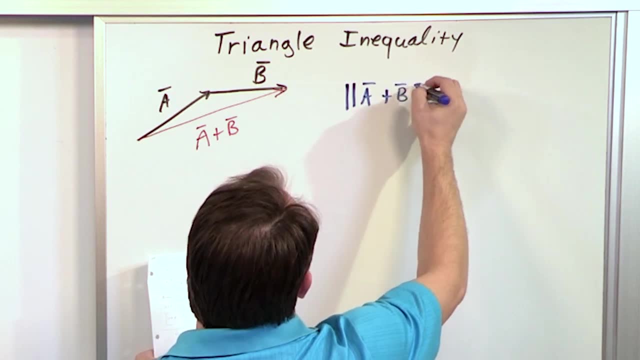 inequality is something you're definitely going to see in your textbook And it's written like this: The triangle inequality says. it looks kind of scary but it's easy to understand. I promise A plus B with magnitude bars around it is less than or equal to the magnitude of A. 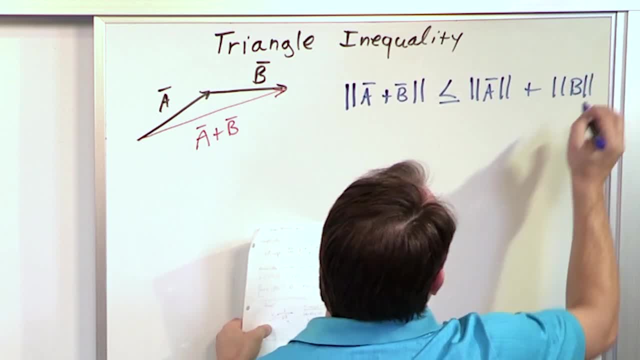 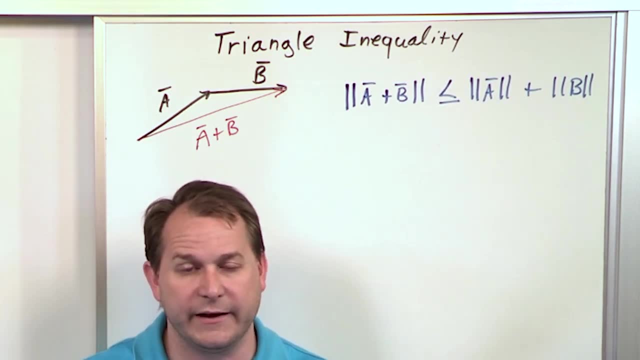 plus the magnitude of B, All right. So people look at that sometimes in a linear algebra book or whatever, and they kind of gloss over it and they're like, yeah, I guess it's right. You know, I guess it's true. Well, I'm going to show you why it's true. It's very, very. 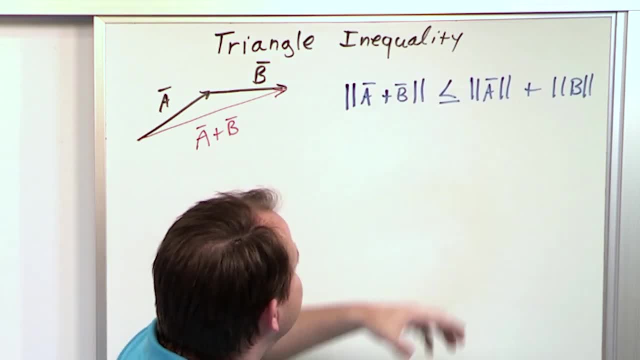 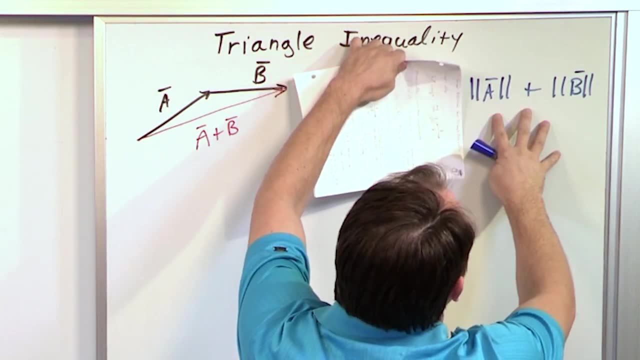 simple to understand. What they're saying is: notice, everything has a vector bar on top of it. I forgot to put the one here. What it's saying is: if you kind of cover this up, all right. just look at this. What it's saying is: you have vector A and a vector B. If you take their. 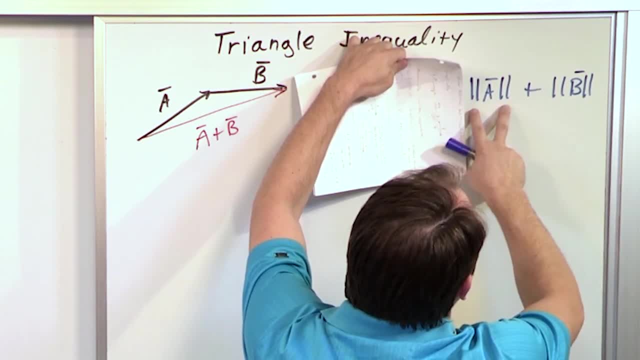 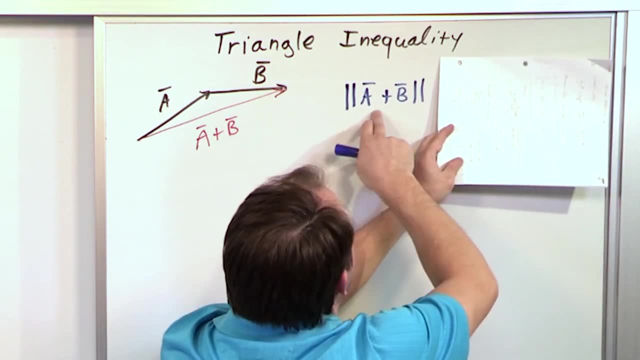 magnitudes and you add them together. So let's say this has a magnitude of five and this has a magnitude of three. You add them up, you're going to get eight, All right. And then you compare that to if you add the vectors first and then take their magnitude, then what you're 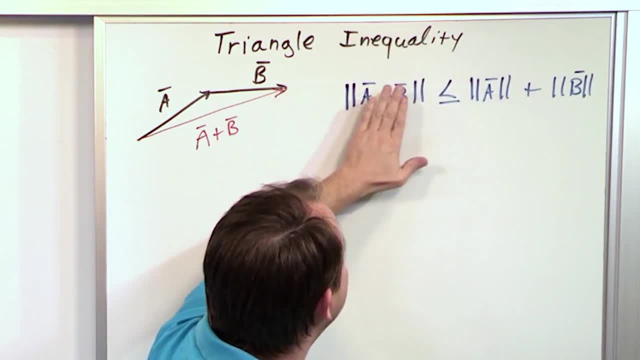 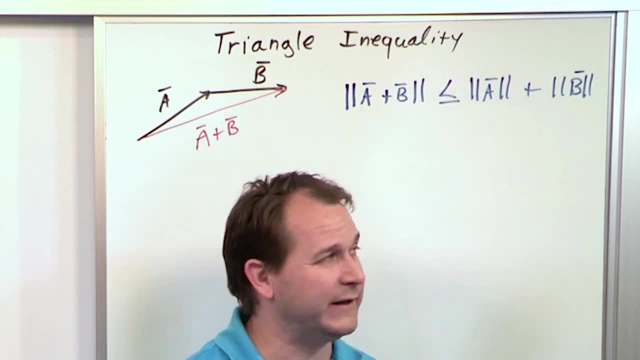 going to get is you're always going to get a smaller number on this side of the inequality. That's why it's pointing this way. Then, if you add the vectors, their magnitude of the vectors, separately, All right, There's also a less than or equal. I'll explain in a minute The reason. 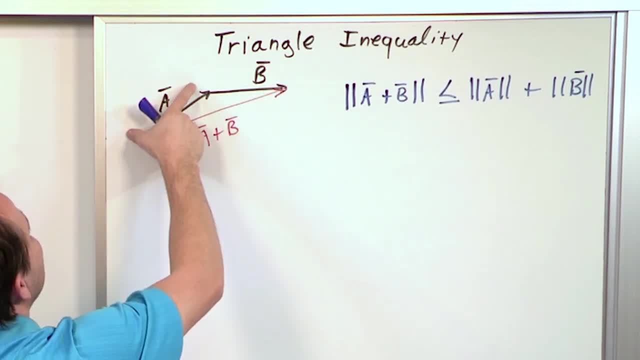 it's called a triangle. inequality is because of what we have here. You see, length of A is represented by this arrow. Length of B is represented by this arrow. Because of the geometry, length of A is represented by this arrow. Length of B is represented by this arrow. 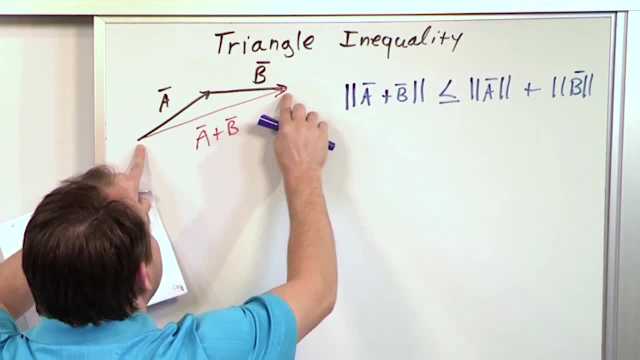 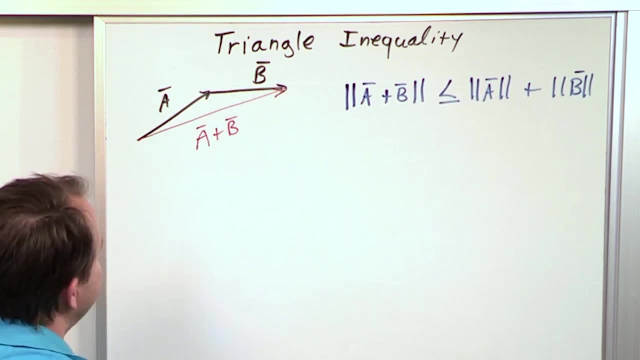 Because of the geometry, what it's saying is the length of A plus B, the length between here. that's what this term is. The length of this is always going to be smaller than if you took the length of A and then separately added it to the length of B, And you can see that from the 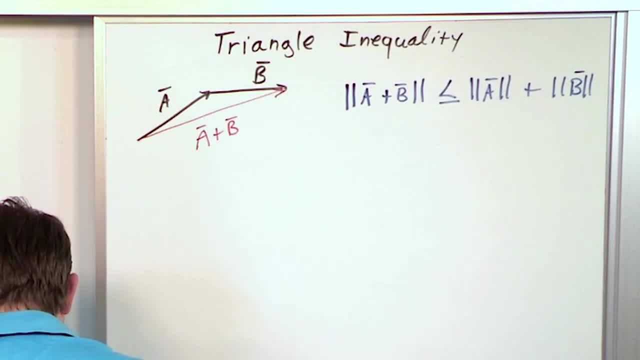 geometry, No matter how you orient A and B. See here's A and B now. No matter how I orient A and B, the resultant connecting those guys as a sum is always going to have a shorter arrow than if you took the length of one plus the length of the other. If you actually got a shorter arrow. 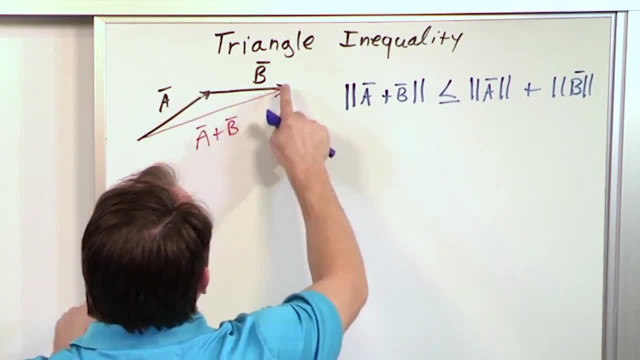 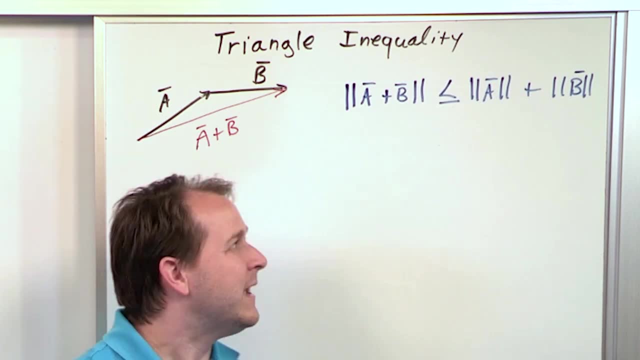 got a ruler out, measured this, measured this and measured this. you would see that when you add the magnitudes here, you're always going to get a smaller number. The only time you're not going to get a smaller number is if A and B actually didn't have an angle here, If A and B were just 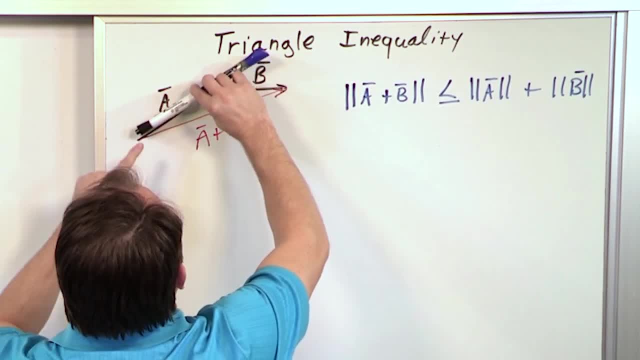 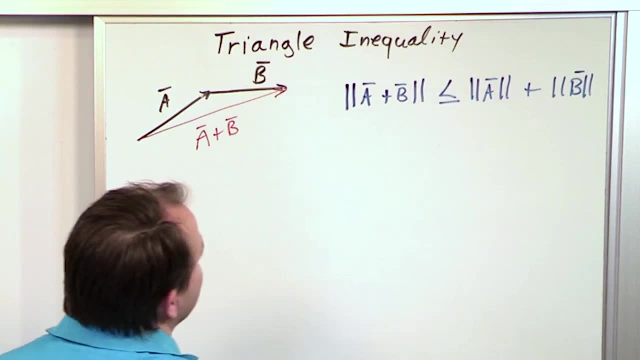 happened to be straight, lined up straight like this, right then the resultant would be the exactly the same as the length of A plus the length of B. That's why there's an equal sign here. So it's always going to be less than or smaller than, if you individually. 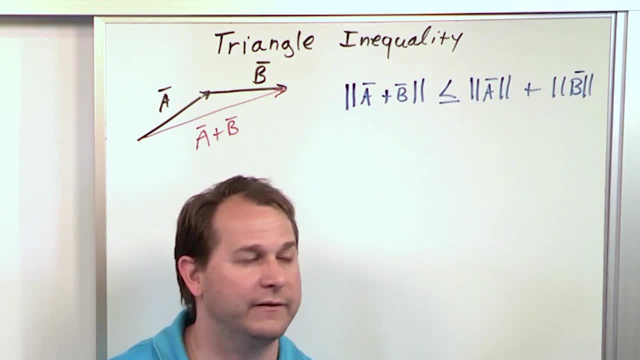 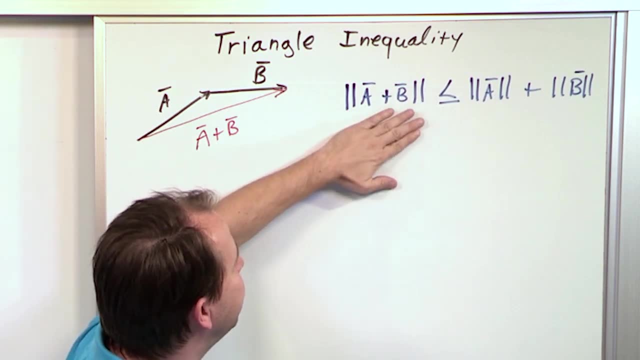 take the magnitudes of the vectors you care about and you're adding up the magnitudes. So what you're doing is comparing numbers: Length of A plus length of B, that's probably going to almost always be bigger than if you take the vector sum and then do the magnitude. 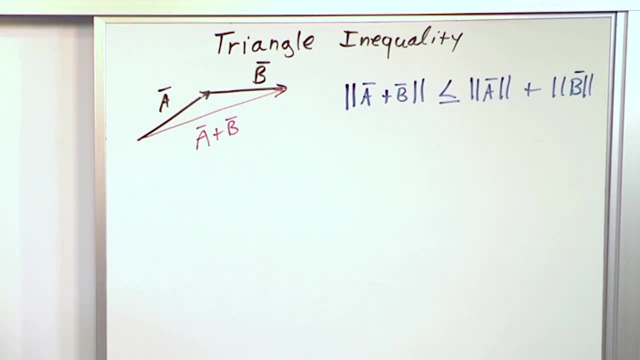 That's what it's basically saying. All right, So that's the triangle inequality. Let me draw a little line here. Now I want to discuss something called the Cauchy-Schwarz inequality, which we'll talk about. But before I can do that, I want to 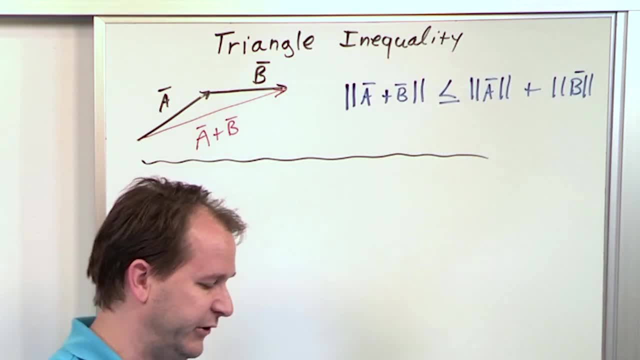 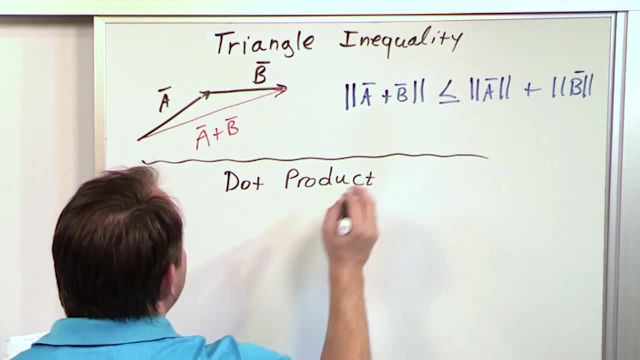 talk a little bit more about the vector dot product that we have discussed so much in the past. So let's talk about the dot product again Now. I know you don't know how to calculate it- We've talked about it several times- but I want to draw a picture. So let's say we 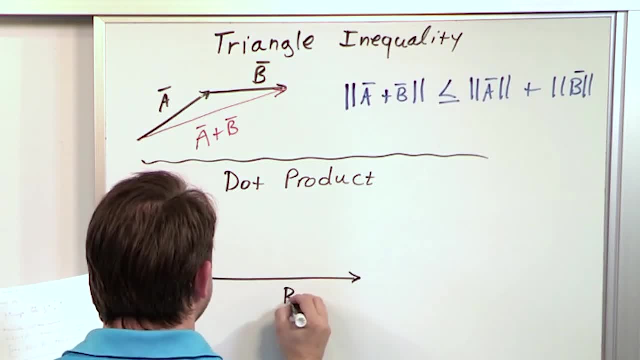 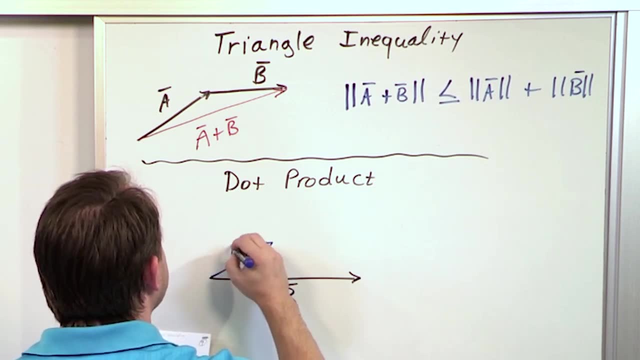 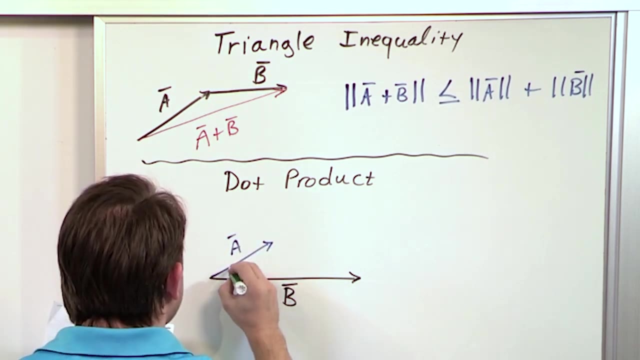 have a vector here and that's called vector B, All right, And then up above we have vector A, like that, And in between them, because the vector A is cocked up with respect to B, there is an angle, obviously, between A and B There. 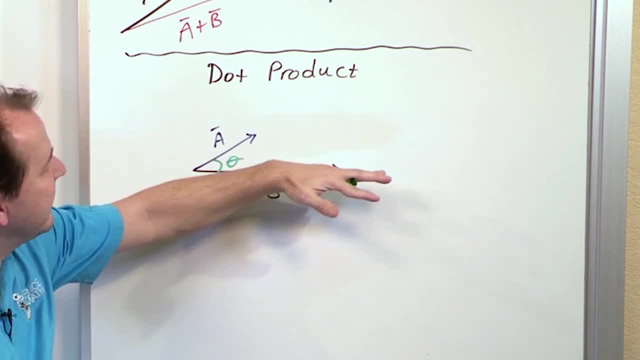 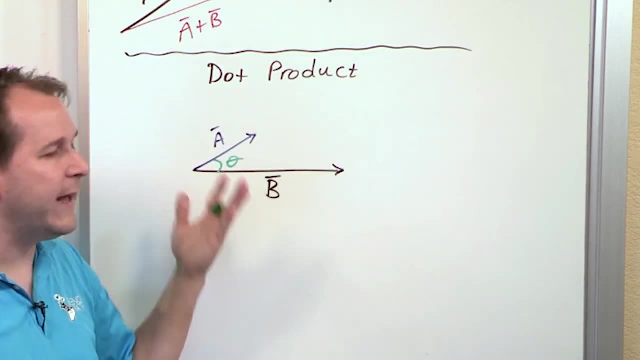 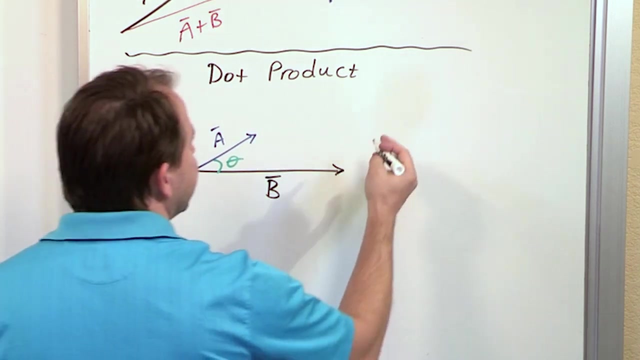 always is, unless the vector A is exactly in line with the vector B, in which case the angle is 0. But at any other time there's going to be a non-zero angle between A and B. right Now, the dot product is something that we've talked about several times. The 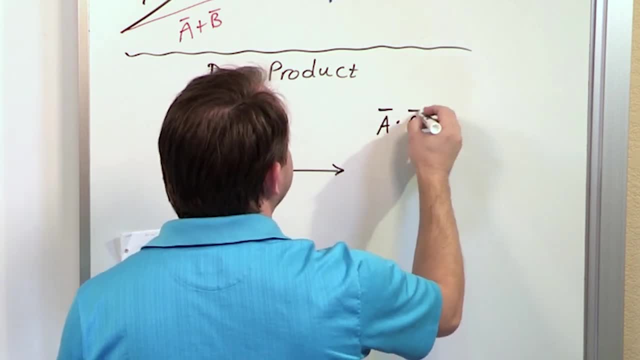 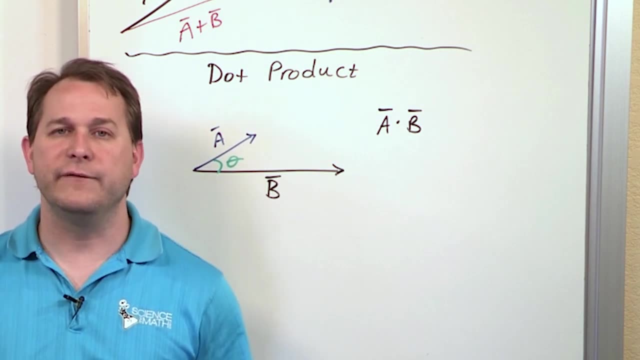 dot product A, dot B. We already talked about it in terms of, you know. we've talked about it in terms of, you know, multiplication, where you multiply the elements of the two vectors and sum the results. We've talked about that. That's one way to calculate the dot product, But another 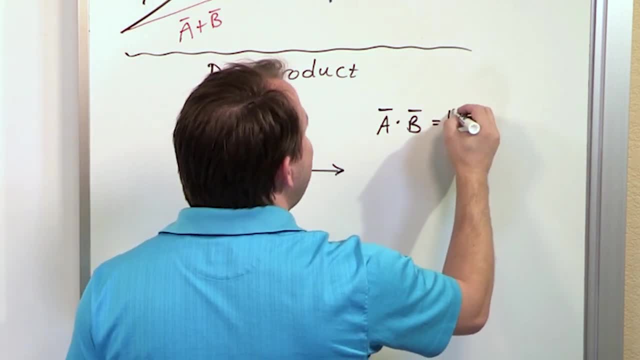 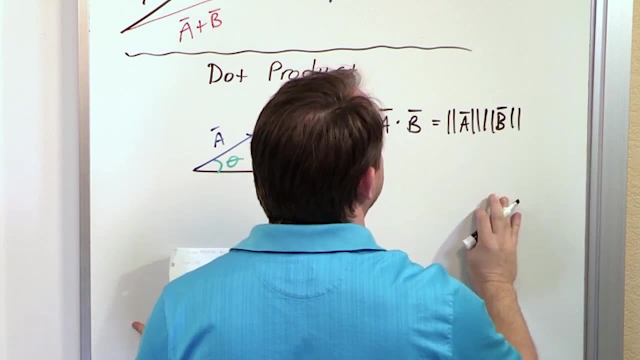 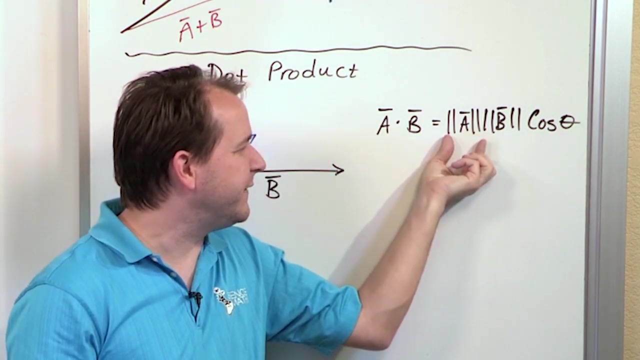 way to calculate the dot product is, you say, magnitude of the vector A right times the magnitude of the vector B times the cosine of the angle between the vectors? This is a definition that you've probably seen in a physics book, but you may not have seen. 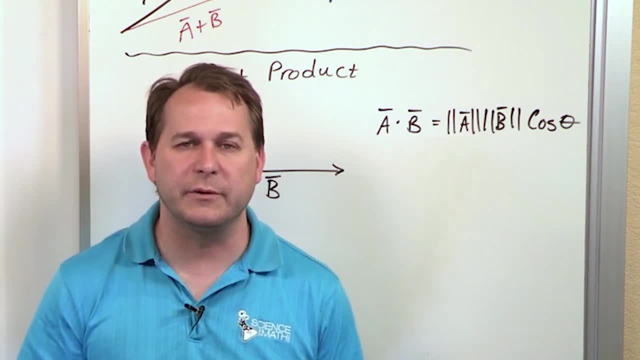 these magnitudes, these double bars. That's kind of something that we're going to talk. you're going to see in a linear algebra class. some other physics books might show it. but the way you read it is, if you're going to dot two vectors together, it's the length of a or the. 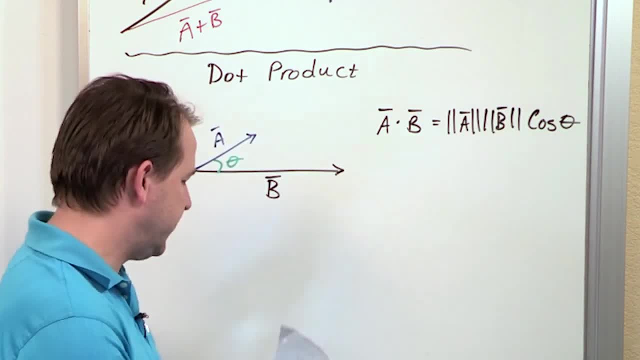 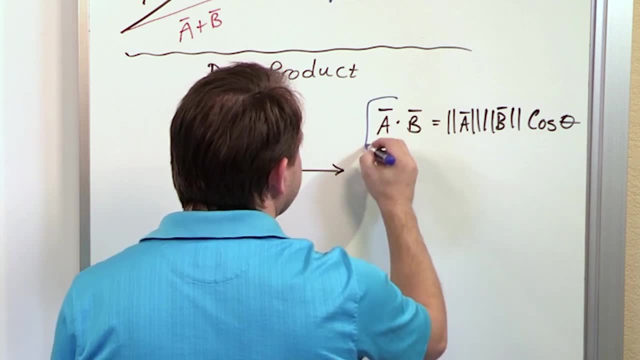 magnitude of a times the magnitude of b times cosine of the angle. Now let me show you something to make this a little bit clearer to read over here. We can rearrange this freely, so let me circle this, because this really is the definition of the dot product. all right, But you can also 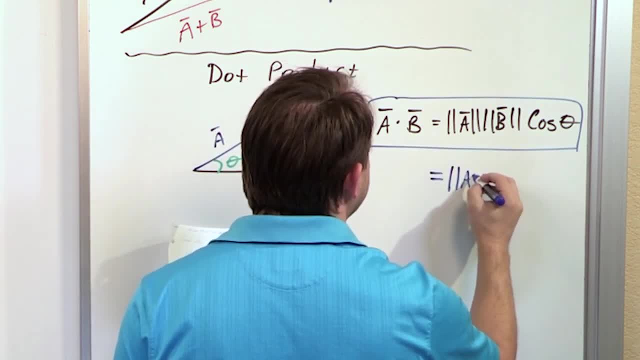 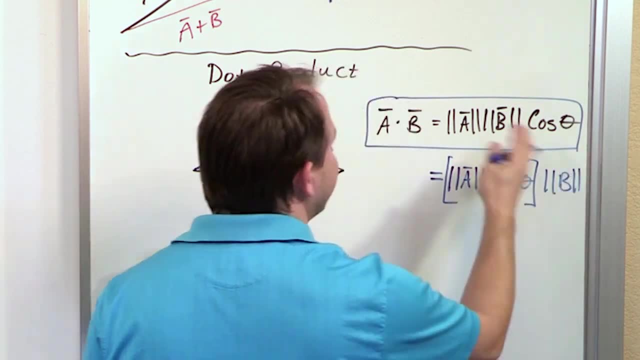 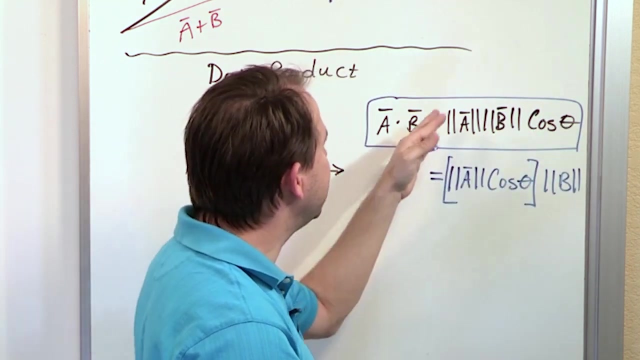 write it as follows: You could say: magnitude of a times cosine of theta, times the magnitude of b. All I did was rearrange the order of the multiplication. I'm multiplying a number, magnitude a times magnitude b times cosine of an angle. So I can freely. 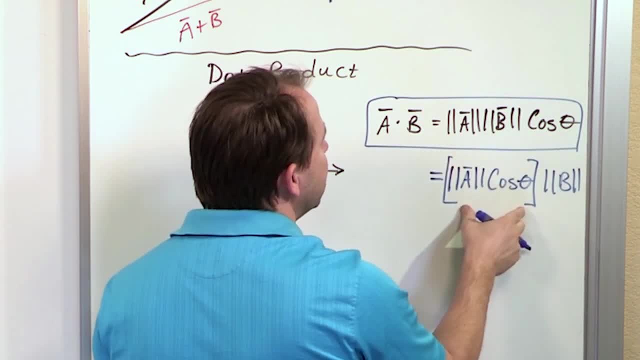 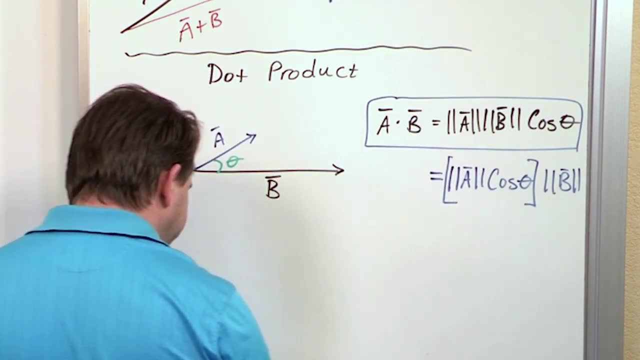 change the order of multiplication. so I'm going to say a times cosine, theta times magnitude of b. all right, And the reason I'm going to do that is because I want to show you in this drawing what is the magnitude of a times the magnitude of b times the magnitude of b. 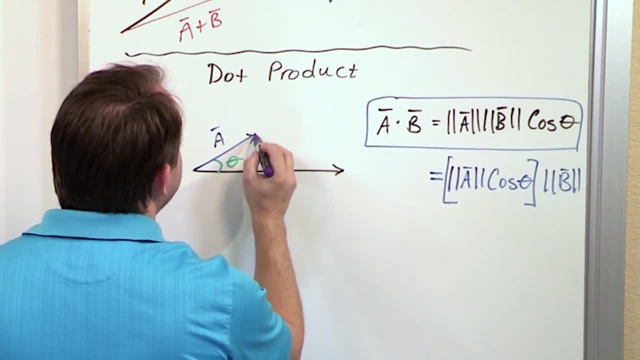 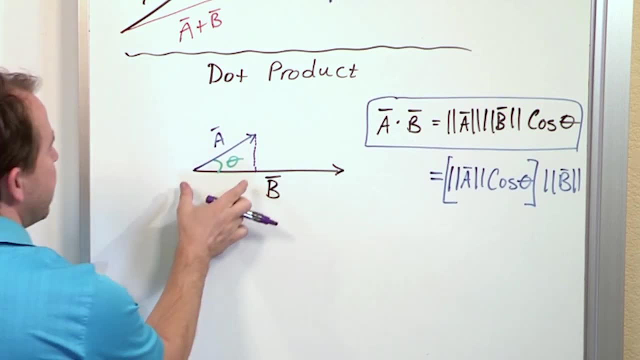 What does cosine do? If you remember back from trigonometry, right, If you take the projection of this vector down to the b line there, then what's happening is this projection down here. this length from here to here is what we call a times cosine theta. You can think of the cosine. 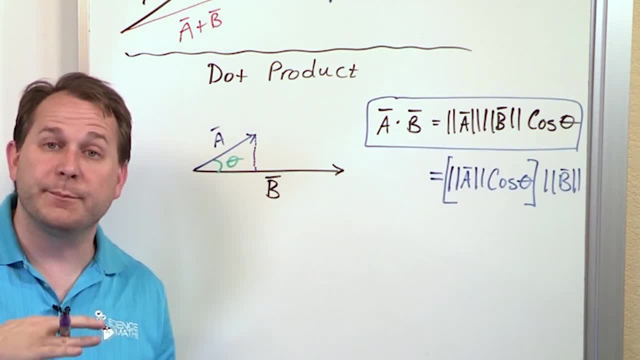 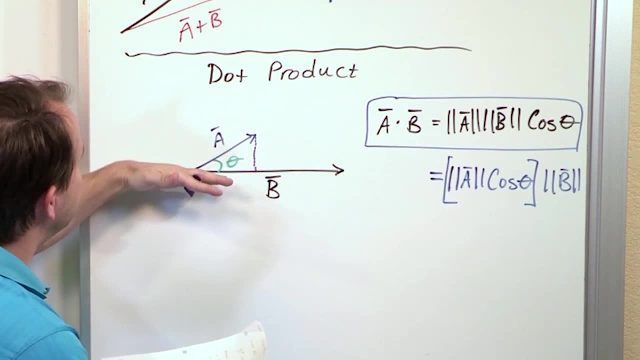 function as chopping the vector and getting the projection along the b vector. So we're looking at two vectors: always when we have a dot product and when we have a times the cosine of theta, we're looking at the component of this vector that falls along the b vector. So if I wanted to, 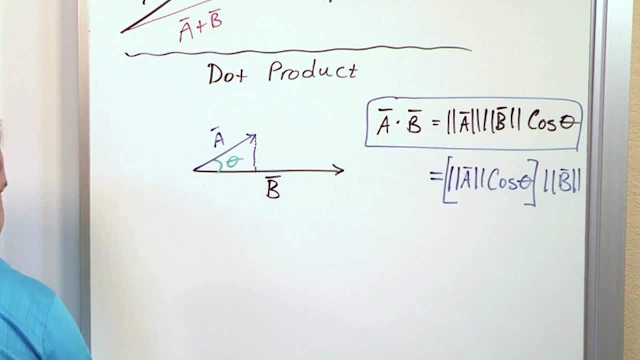 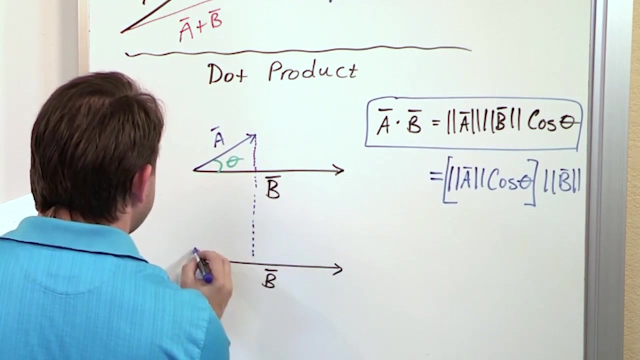 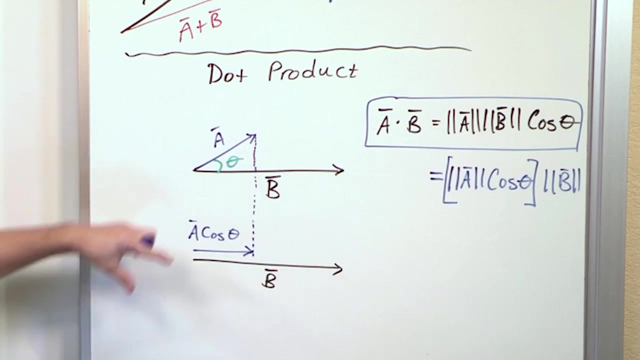 redraw it just to make it a little bit clearer. let me use the same colors to make it a little bit clearer. Then, if I'm going to do my dot product, this is b again, right. And if I line everything up perfectly, this distance is what we call a cosine of theta, right? 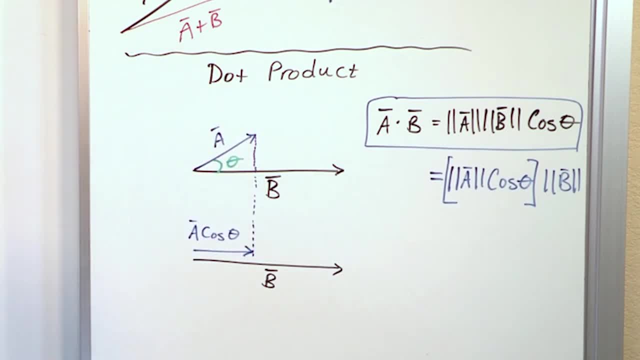 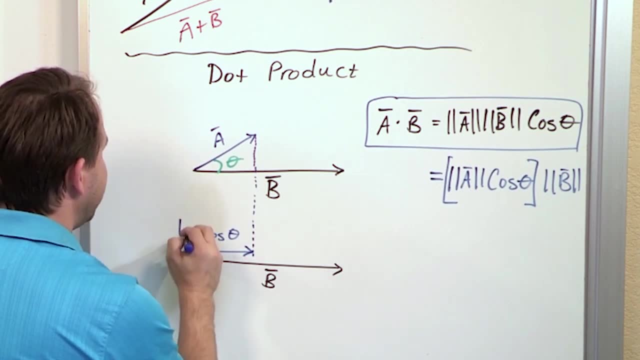 So it's this length from here. It's chopping it and getting that projection down. So we take a cosine theta and it's actually magnitude of a cosine theta. So let me put that there. Magnitude of a times the cosine of theta, That's the length of this arrow, all right, And then we're multiplying. 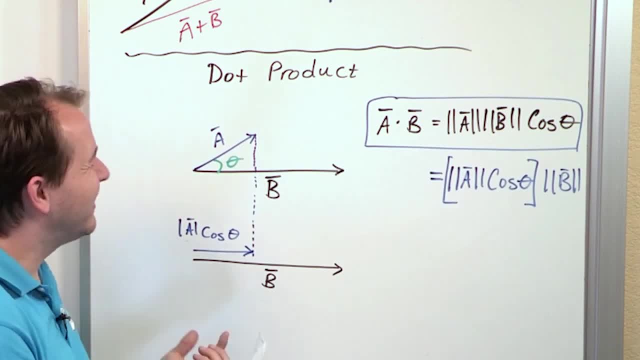 by the magnitude of b. What we're doing when we calculate the dot product really is, we're seeing, we're trying to multiply the vectors together, But really all we're interested in doing is multiplying how much of a falls in the b direction, and we're going to multiply this length of this. 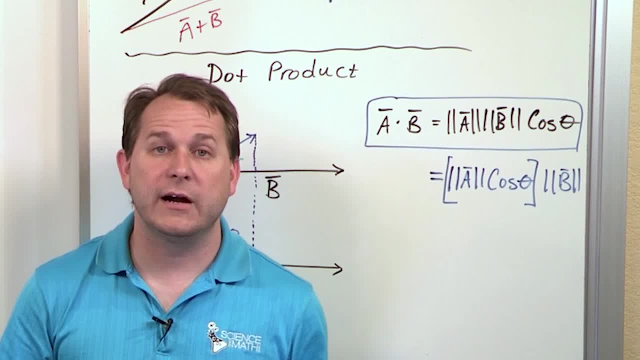 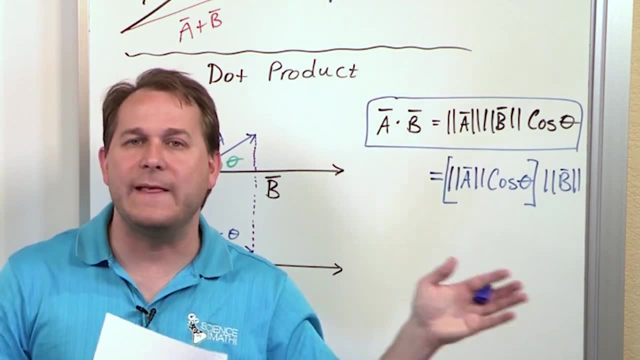 arrow times the length of this arrow. So you can think of vector dot product as basically trying to multiply the vectors. but we only care about how much of a falls in the b direction and that's what we multiply times b. all right, So back in physics you learn about work That's force dotted. 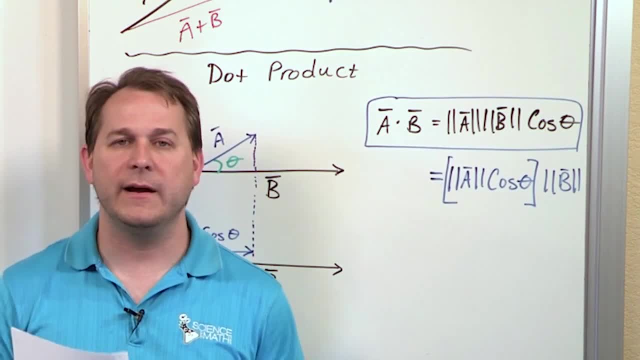 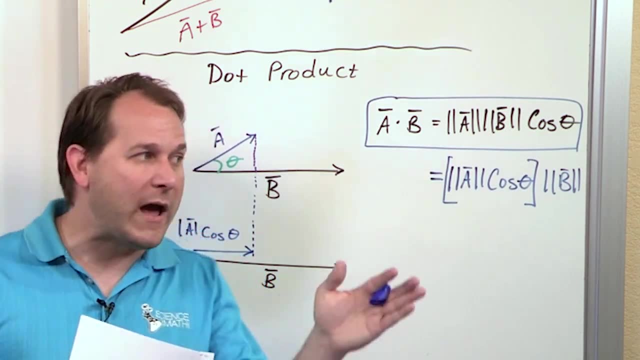 with distance. Whenever you're calculating work, you only care about the amount of the force that is in the direction that you push the object Force dotted with distance. So the dot product is a way of chopping the force down. If you have an angle with your dot product, you're going to 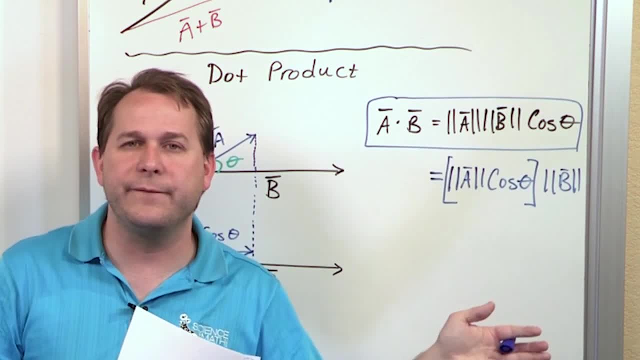 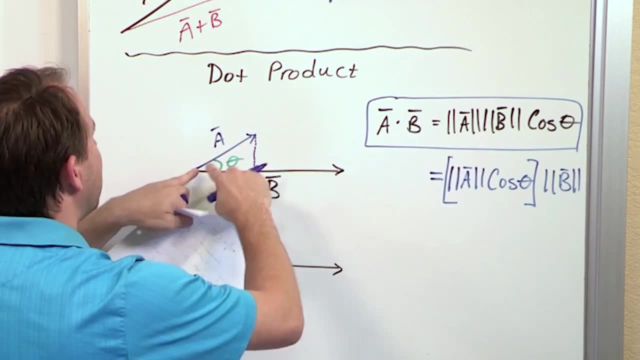 be chopping that force down to only get the component of that force in the direction of motion. That's what we're doing here. So you can think of b might be the distance I push a shopping cart and a might be a force vector I'm pushing on a rock. If I care about the work done, I'm going. 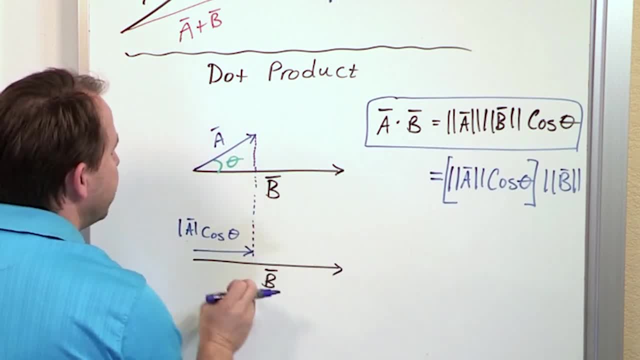 to chop it down, get the component of this force that falls in the direction of motion, and I'm going to multiply these things together. That's why the dot product is defined in this way. all right Now, of course. I'll circle back and remind you, though, that 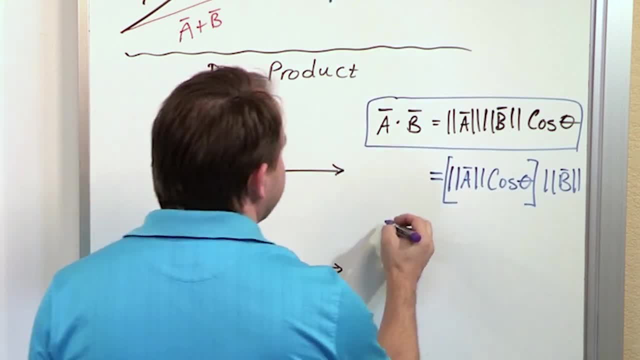 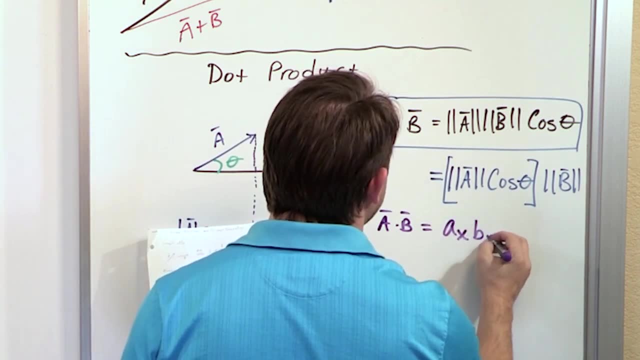 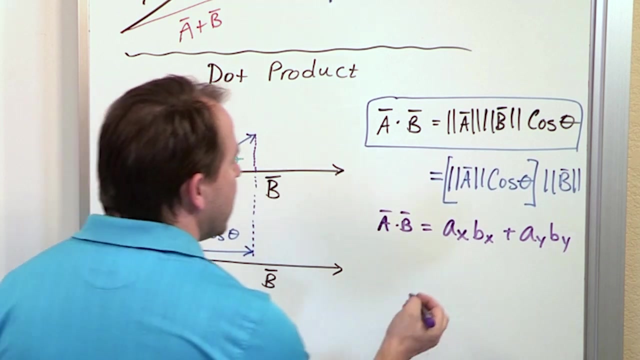 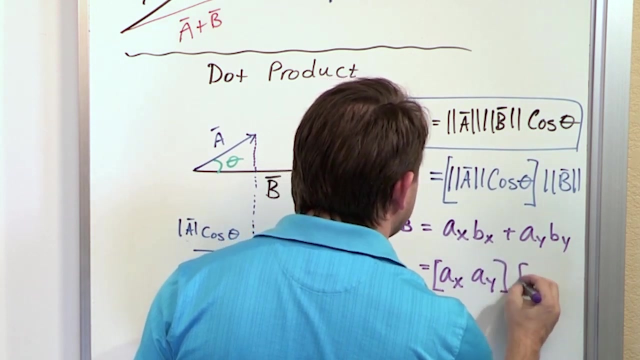 we have also been calculating a dot b in terms of components, right? We can say a sub x, b sub x, plus a sub y, b sub y if it's an xy vector, right? Which is exactly the same thing as saying a sub x, a sub y, b, sub x, b sub y. This is the dot product in terms of. 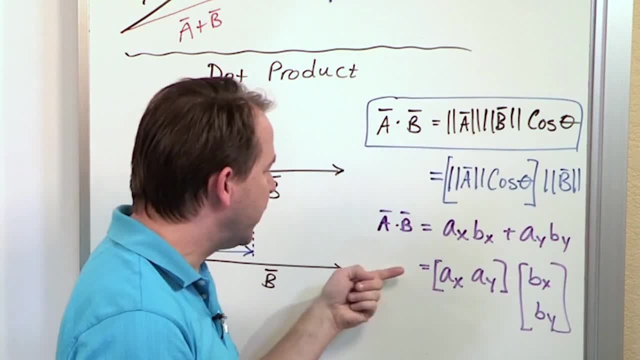 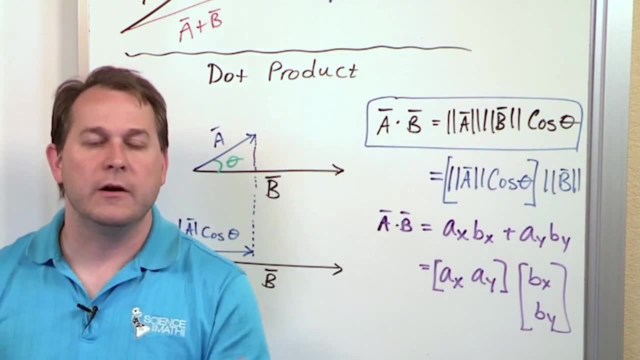 uh matrices. So if I know my a vector and I know my b vector, I go across and then down. So basically, all I'm doing is multiplying the x components of the vectors together, I'm multiplying the y components of the vectors together, I'm adding everything together. I get one number as: 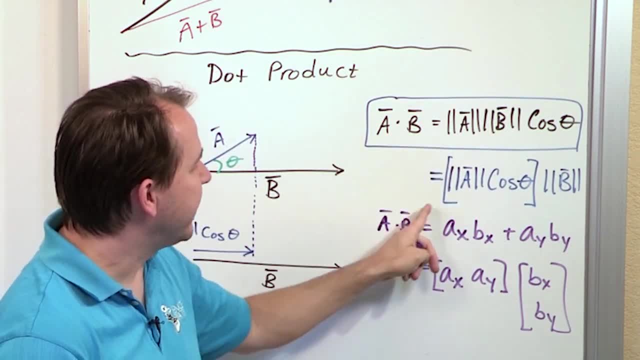 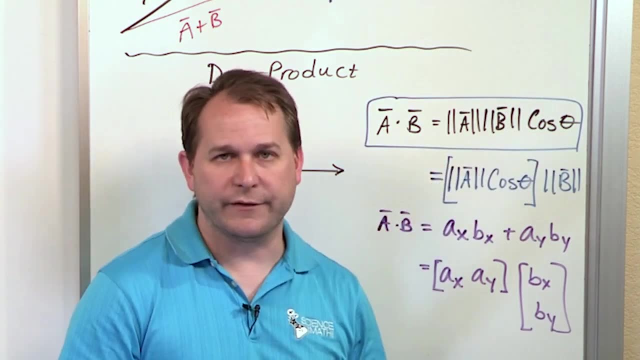 a result of the dot product. Notice, it's completely consistent with this. I get one number as a result of this calculation. I get also get a number here. This is a number, This is a number. Cosine of an angle is also a number. So I just arrive at a number for the dot product. So basically, there's. 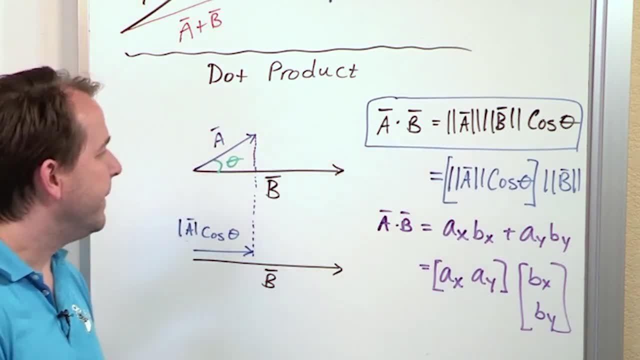 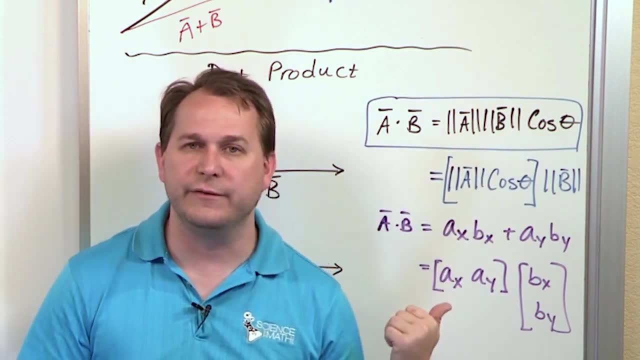 two ways to calculate a dot product is the bottom line Um. number one. you can do it in terms of components. Number two: if I know the magnitudes of the vectors and the angle between them, I can use the other relation. They both give the same. 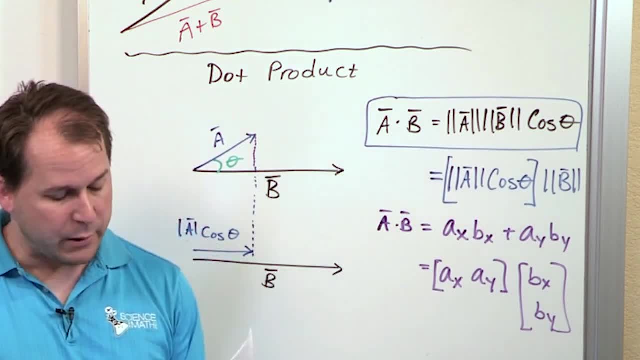 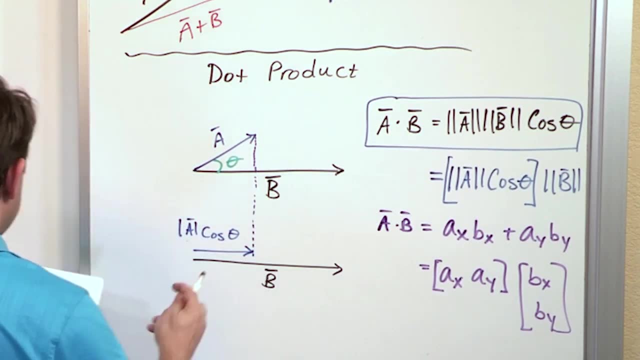 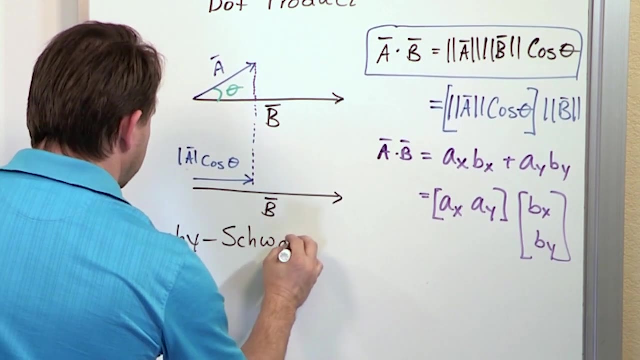 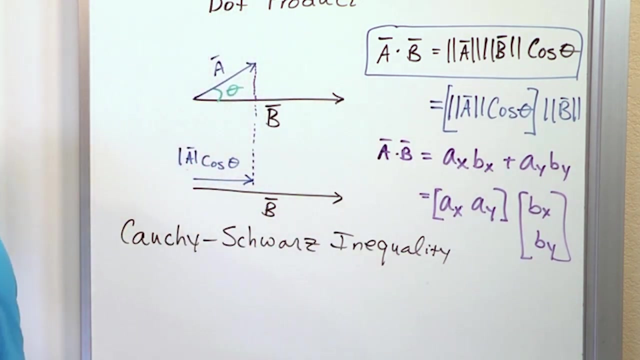 answer. Your dot product is going to give you the same thing between both of them. Now I wanted to cover this because we're going to be learning about something called the- uh, Cauchy Schwartz inequality, And, without further ado, I'll go ahead and put that on the board. And now that we've done a little, 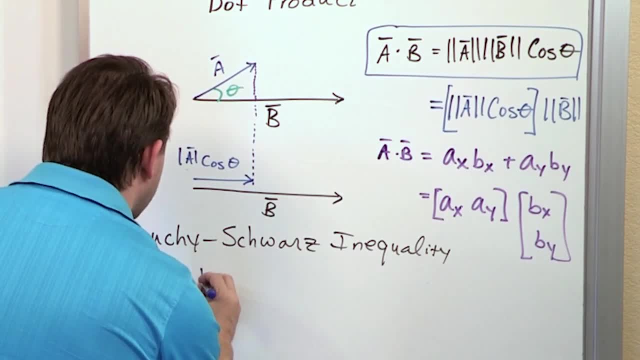 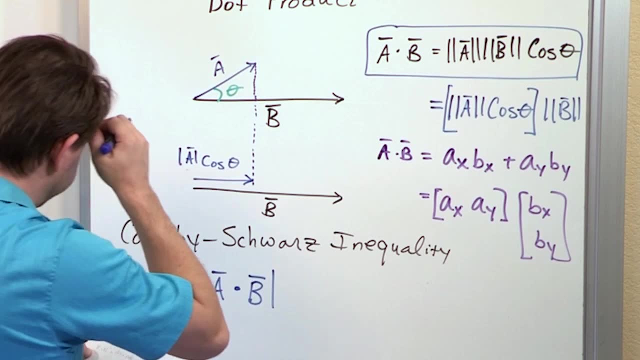 review of dot product, you'll understand exactly what it is. The Cauchy Schwartz inequality says that if you take a vector a and you dot it with a vector b and then you take the magnitude of the result, that it's going to be always less than or equal to the magnitude of a. 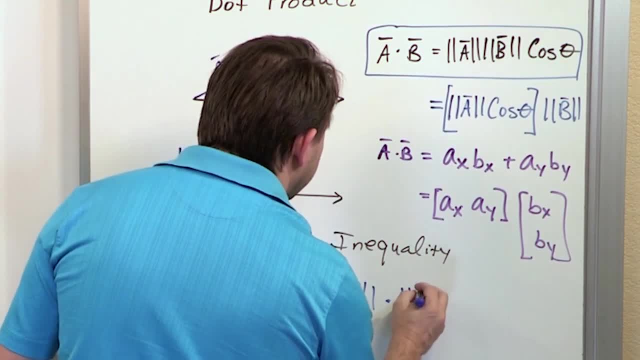 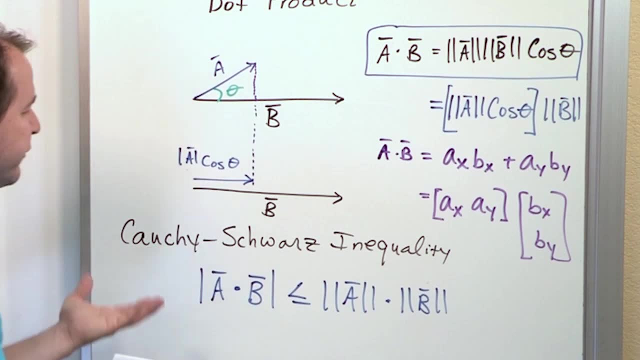 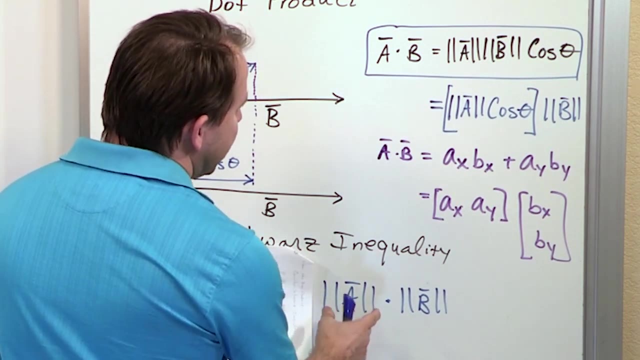 multiplied by the magnitude of b. So it's very similar to the triangle inequality in terms of its form, And you can understand what it means by now looking at this picture that we've constructed on the board, What it's basically saying if you look at just this side of it here, if I take the 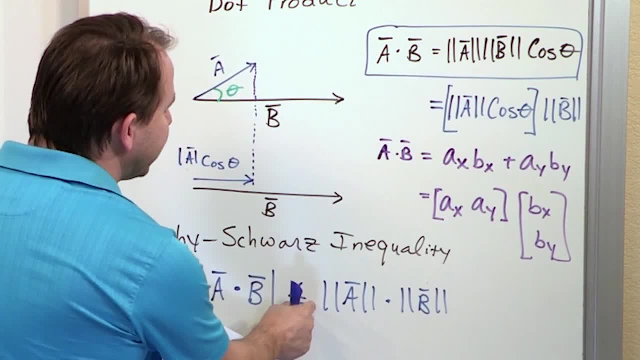 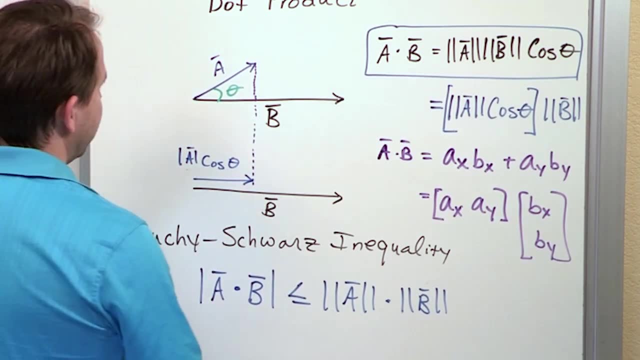 length of vector a and multiply it by the length of vector b, that's always going to be bigger than if I take the dot product and then just look at the absolute value of the result And you can kind of see that from here. Basically, if, if you look at this particular case, you have an angle between 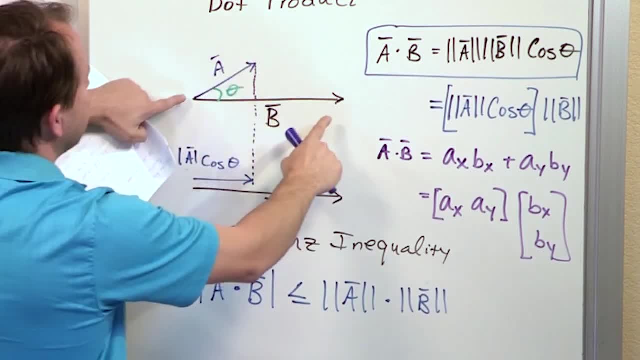 a and b. All right, The length of a is this. the length of b is this. So, if I take the length of a times the length of b, that's the length of a, And if I take the length of a times the length of b. 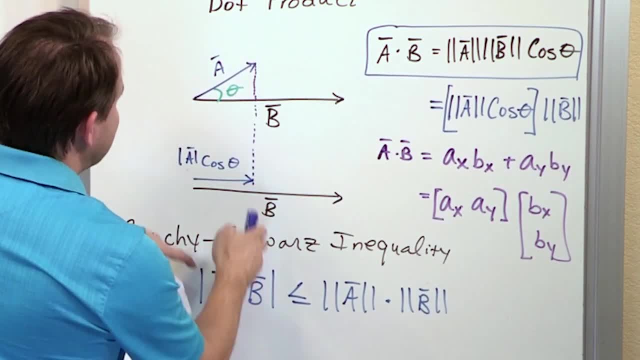 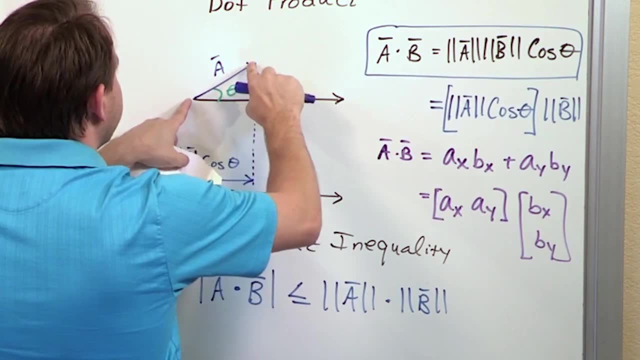 that's what I've got on the right hand side. But then when I take the dot product, I'm always chopping this vector down. So the length of this chopped version in the direction of b is always going to be smaller than this. So this arrow here is always going to be smaller than the magnitude. 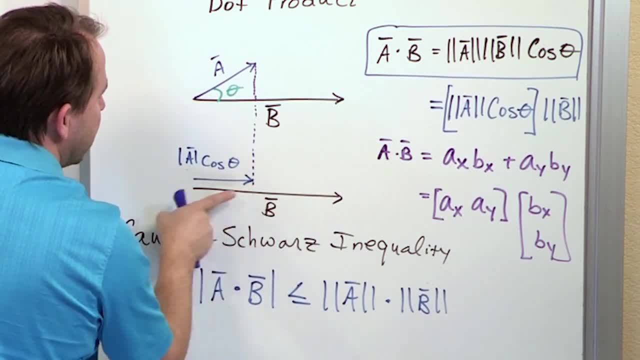 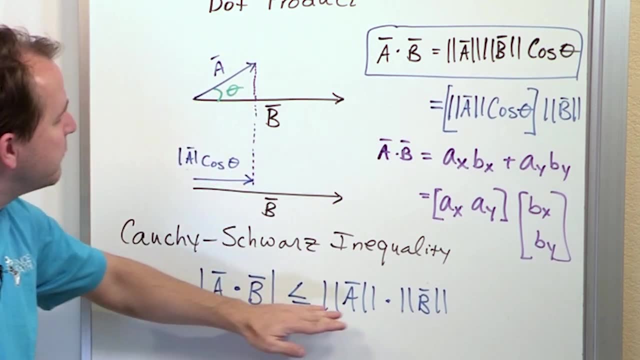 of a, because I've chopped it and I'm only looking at the direction of a, or the vector a in the direction of b. So when I take the dot product like this of the two vectors, what's inside of here should always be smaller than if I multiply the magnitudes of the vector separately, because 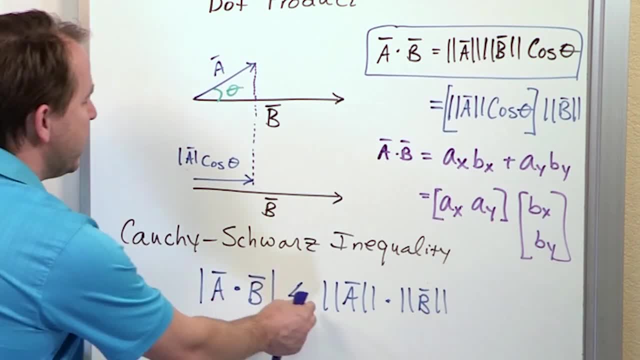 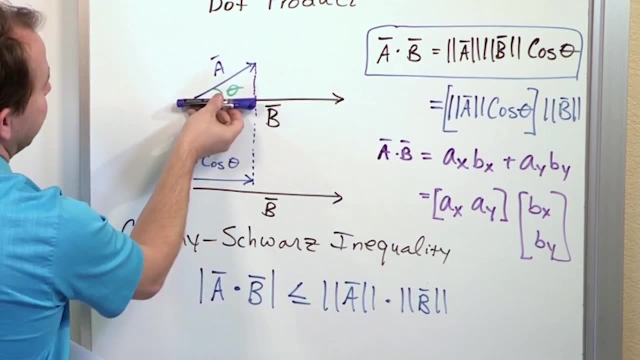 of the fact, of the geometry here, The only case in which it would be equal is if the vector a already was in the direction of b. So so beta is basically, theta is zero. So in that case vector a falls exactly in the direction of b, And then when I, then I'm going to get an equal, equal sign on both. 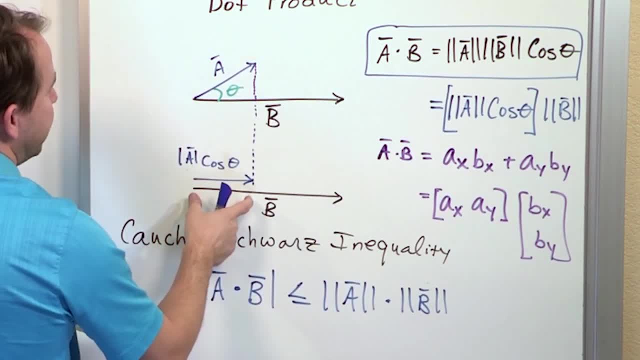 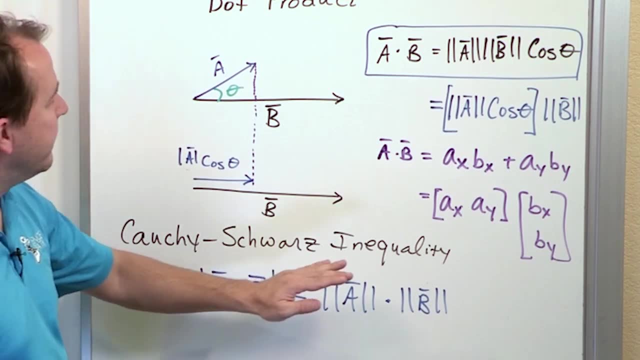 sides, because a times b will be here, A dot b will be the exact same thing, because the vector will already fall along b. So this is the Cauchy-Schwarz inequality there, And it's it's, if you understand the definition of it from what I've described here, from my pictures on the board. 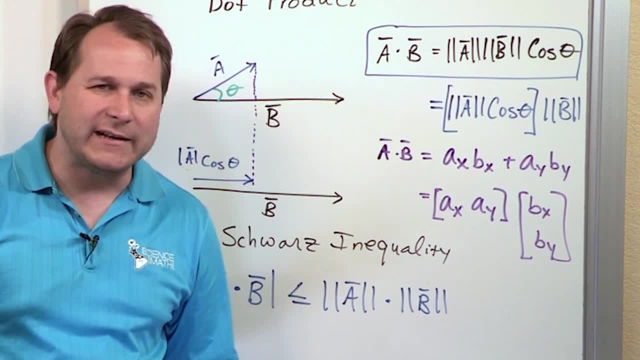 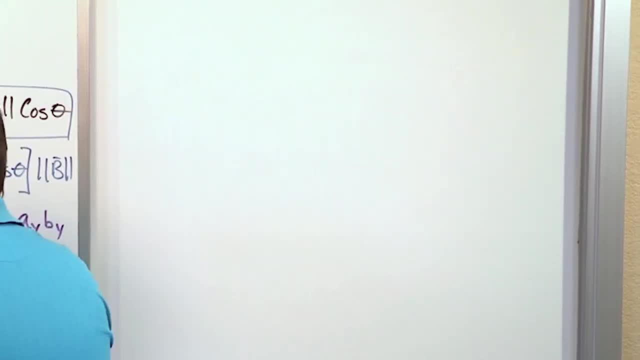 wonderful. that's what I want Mostly. you need to know how to use it, understand kind of basically where it comes from. So we're going to do a quick problem or two to verify that, to to show that that's true. So what we want to do is say, let's say we have vector u and that's going to be 1,. 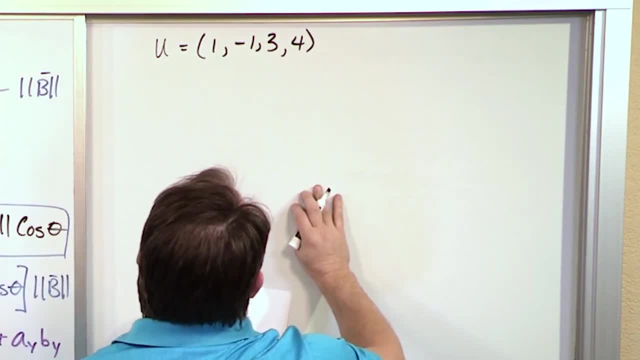 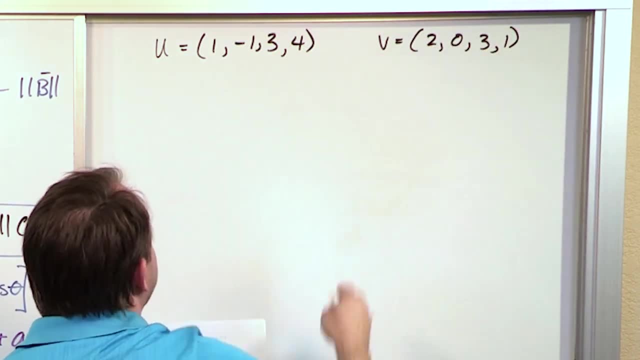 negative 1,, 3, and 4, right And vector v: 2,, 0,, 3,, 1.. Again, we're not in three-dimensional space. here We have four numbers, So this is four-dimensional space. 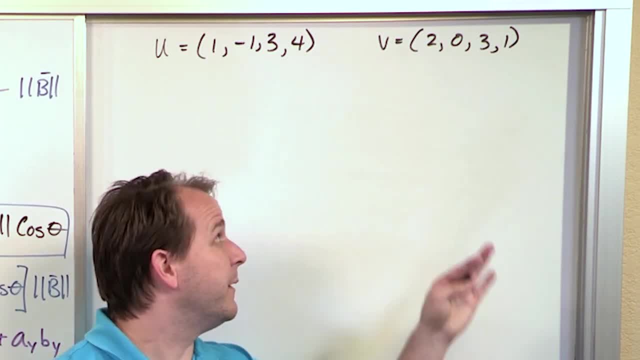 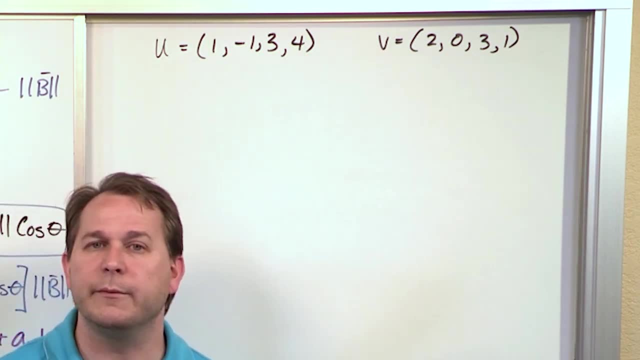 This could be space-time- We're the fourth dimension time- Or it could be some other: temperature, pressure, density, whatever else is in your space that you're considering other than position. It could be any number of things, But in any case, abstractly, your vector has four dimensions for each. 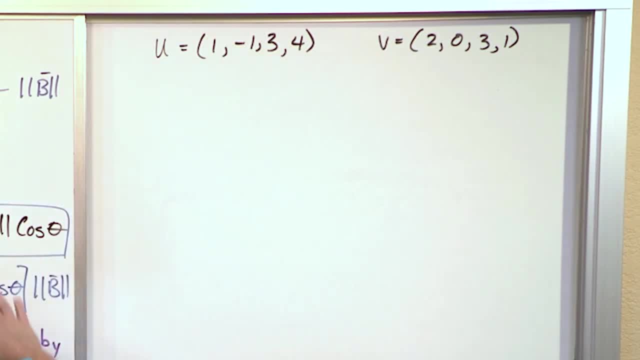 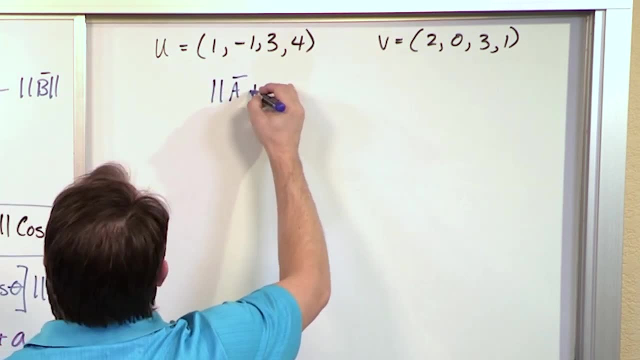 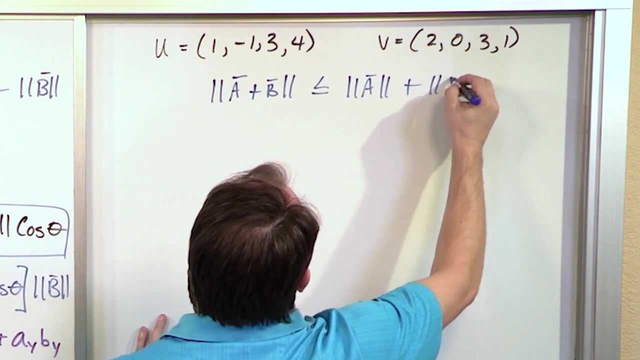 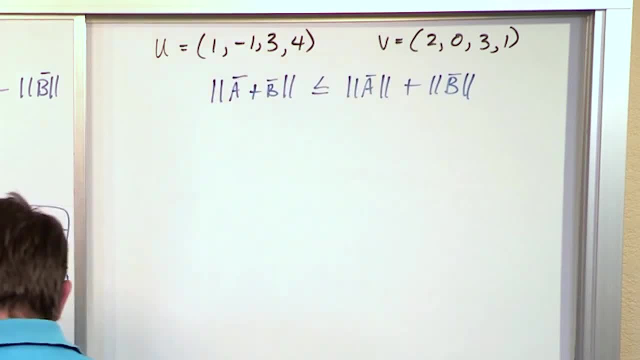 All right. So where a and b are just my two vectors I have. So let's go ahead and do that real quick. First of all, let's find the magnitude of each of these vectors. So the magnitude of u is the square root. 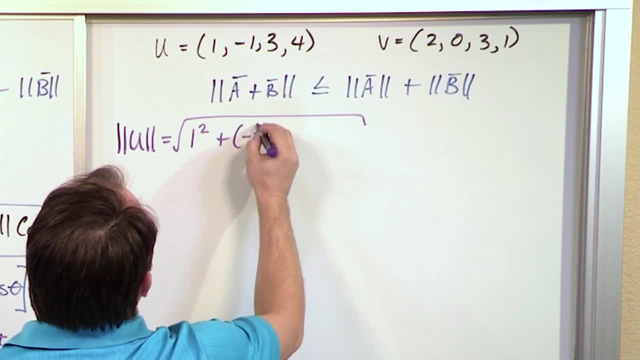 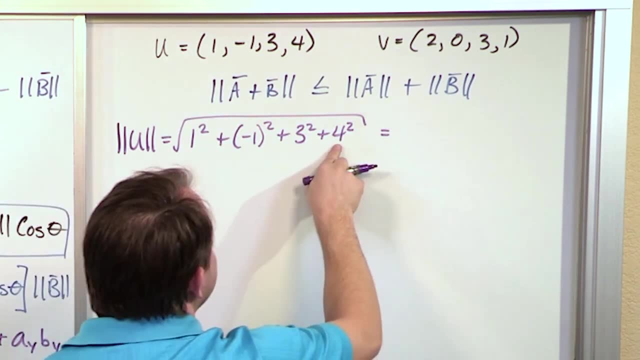 of this guy. here We'll have 1 squared plus negative, 1 squared plus 3 squared plus 4 squared. How many are there? 1, 2, 3, 5, and then inside here, when we add 16 plus 9 plus 1 plus 1, we're going to get the 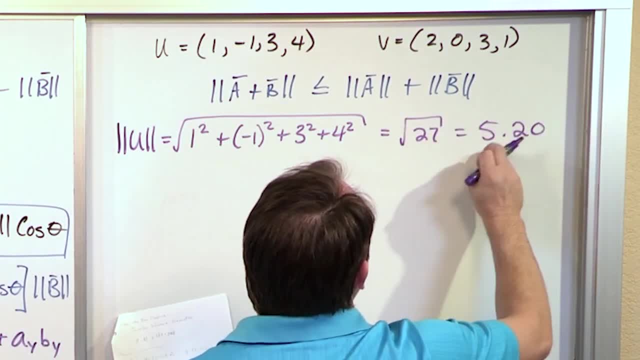 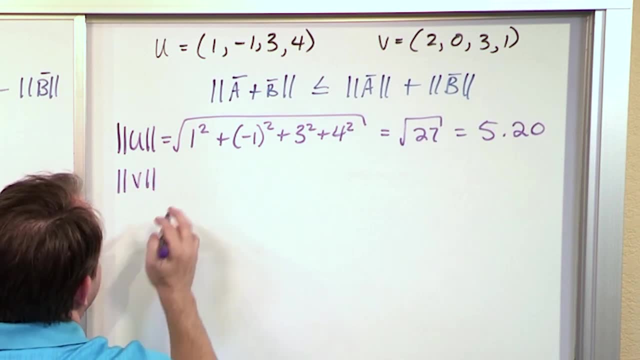 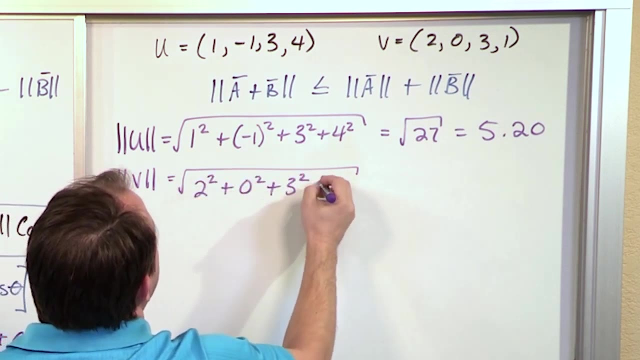 square root of 27, which is going to be 5.20.. I'm just going to move it in terms of decimals so we can do a direct comparison. Now, the magnitude of the norm of v is going to be the square root of this guy here: 2 squared plus zero squared plus 3 squared plus 1 squared. 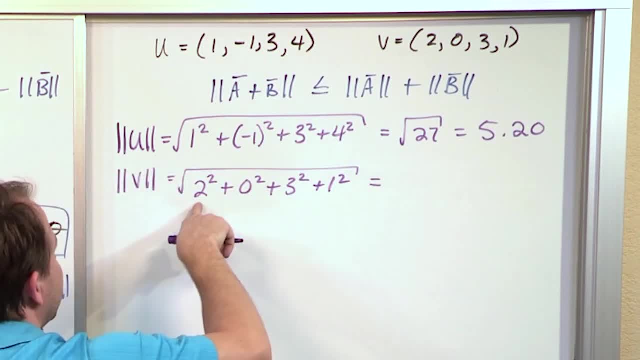 So here we have: 9 plus 1 is 10 plus 4 is 48.. So a root 6 times 10 plus 8 is 10. square root plus 3, squared plus 4 is 14.. So we'll have 14.. And if you take the square root of 14, you'll get 3.74.. 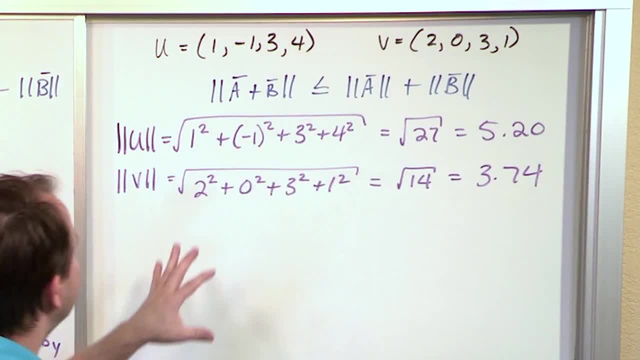 Again just getting decimals so that I can do a nice comparison. So what we have here is basically the right-hand side. We can calculate easily by adding these two numbers together. but let's work on the left-hand side. To get the left-hand side first, we have to add the vectors together. 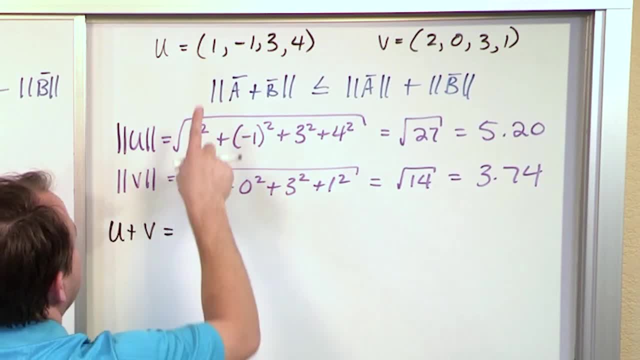 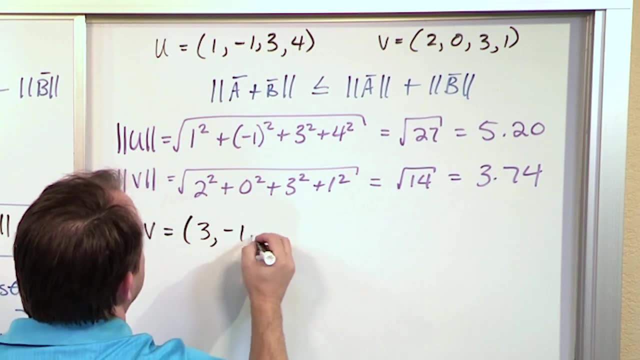 So now we add them, u plus v, And to add vectors we add the respective components. So we'll have: 1 plus 2 gives me 3. Negative 1 plus 0 gives me negative 1.. 3 plus 3 is 6. And 4 plus 1 is 5. So 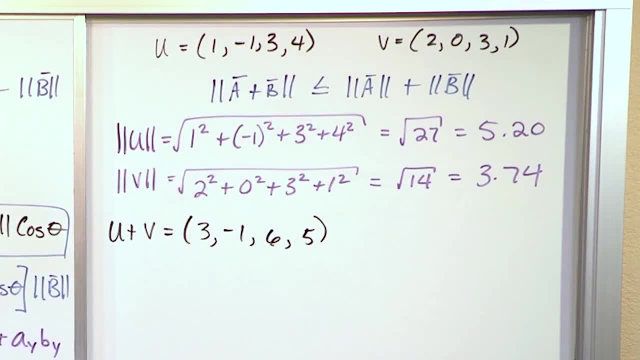 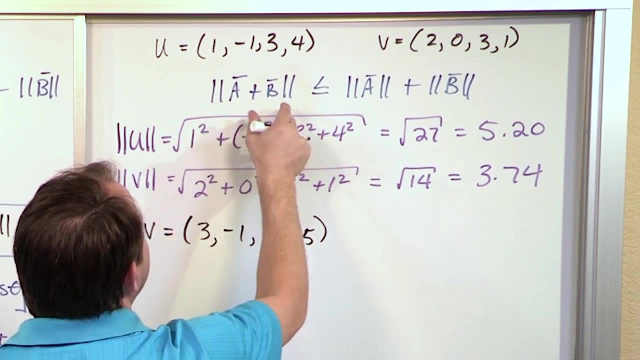 we have 3, negative 1,, 6, and 5. So we just add those two vectors together And now we want to find, because of the triangle, inequality. we need to find the magnitude of what we got as a resultant. 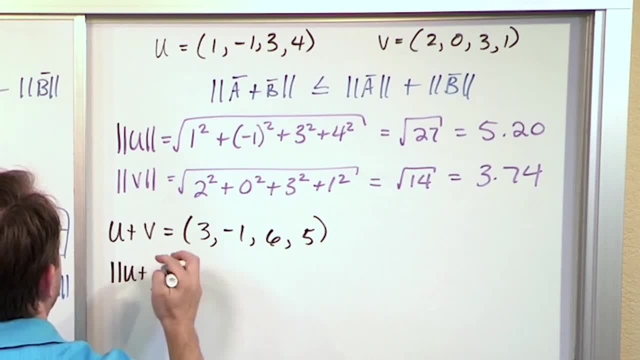 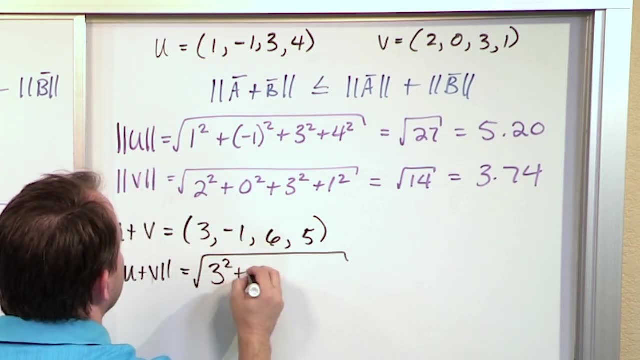 So we'll do the magnitude of u plus v like that And that's going to be the square root of the component. Square root of the component squared: 3 squared plus negative 1 squared plus 6 squared plus 5 squared. We're just taking the square root of the squares of each of those guys added together. 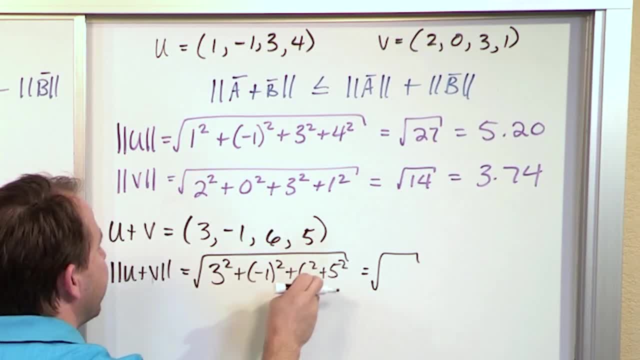 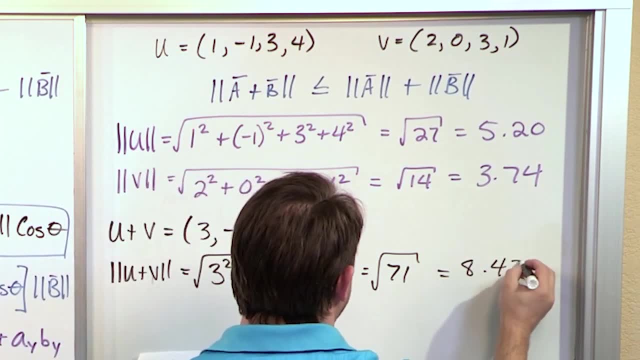 That'll be the square root. If you take 3 squared, this squared, this squared, this squared, add them together, you get 71.. And you'll get, when you take the square root of that, 8.43.. 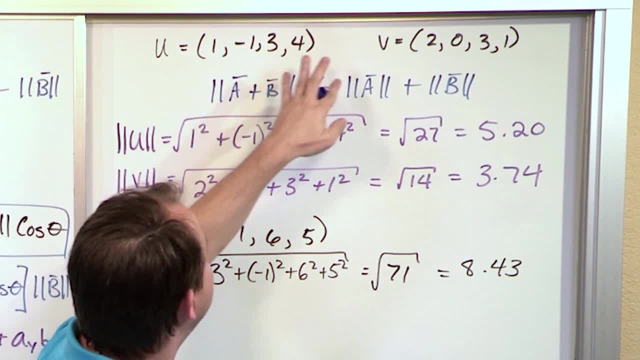 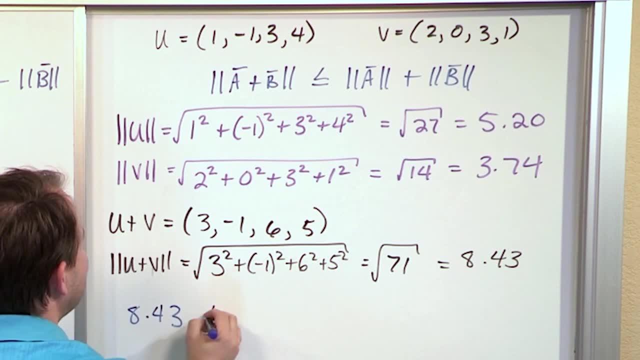 8.43.. So now we're in a position: We have all of the pieces of the triangle inequality. So the magnitude of 8.43 is the magnitude of the triangle inequality. So we're going to find the magnitude of a plus b should be 8.43.. We're claiming that that should always be less. 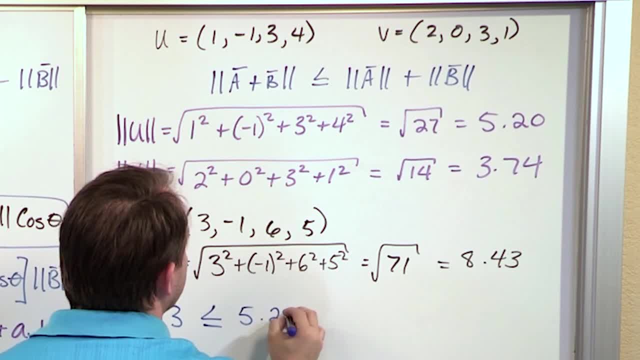 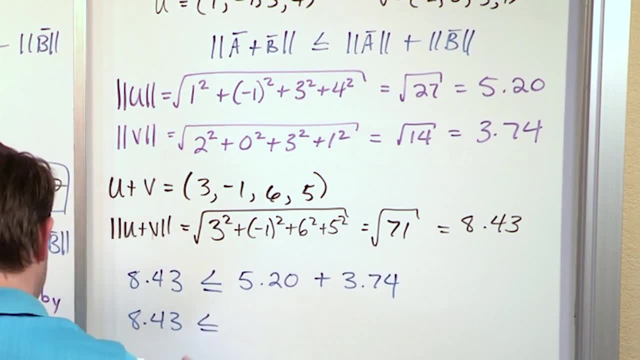 than or equal to the magnitude of a 5.20, plus the magnitude of b- 3.74.. So 8.43, less than or equal to. when you add these guys together, you're going to get 8.94.. So in this particular case, 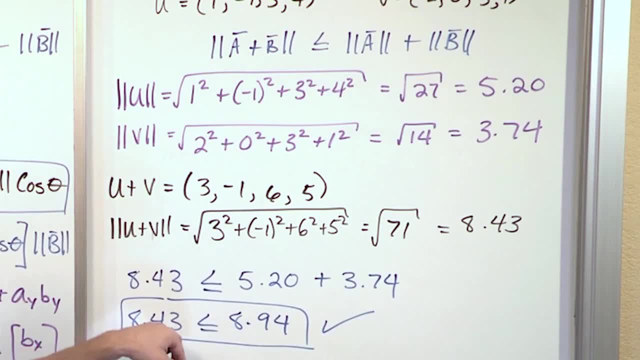 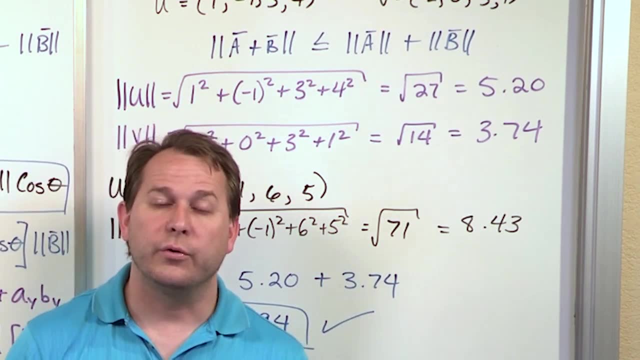 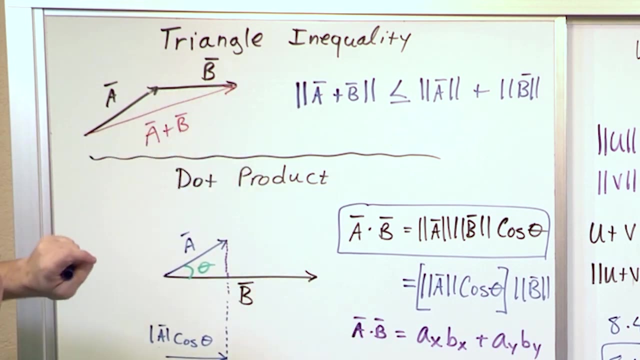 the triangle inequality is satisfied Because when we take the magnitude of the vector sum, we get a number that's less than the individual magnitude of the vectors added or summed together. That's what the triangle inequality is saying. It's saying when you add vectors together, when you add their magnitudes, you're always going to. 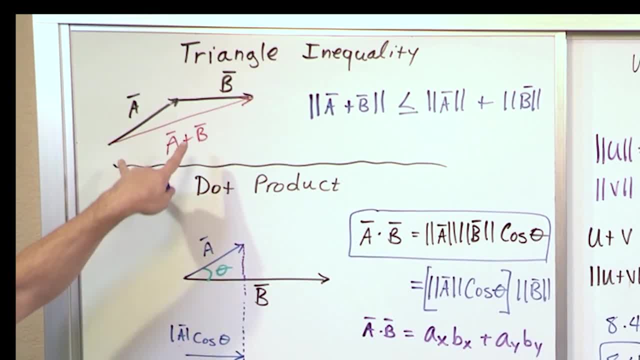 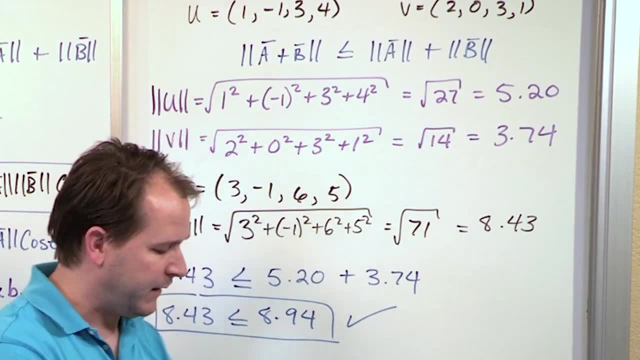 get a number on the right-hand side of this guy bigger or maybe equal to the vector sum. This is the graphical way of understanding it. This is the numerical way of proving that it's true. So you may be asked to do that. All right Now, along the same lines, we want to. 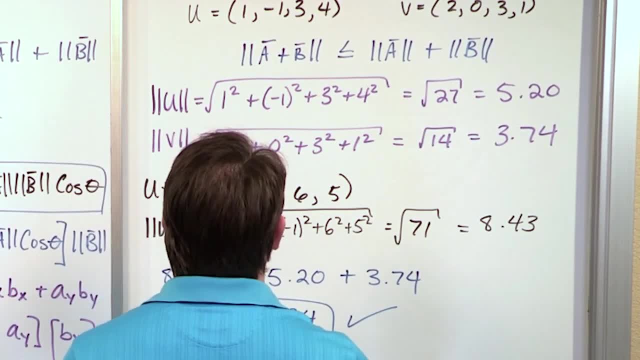 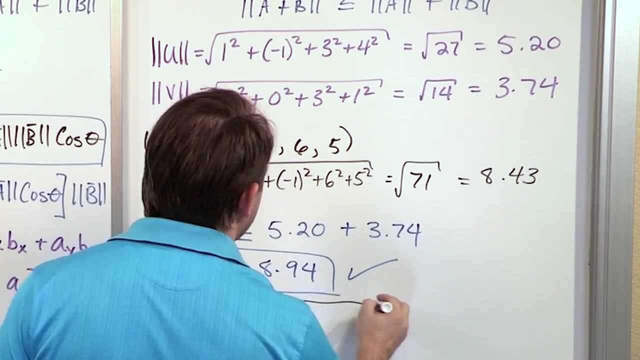 for the same vector. you know, I'll just stay on this board For the same vector. we want to verify the Cauchy-Schwarz inequality. Cauchy-Schwarz inequality. So for the Cauchy-Schwarz. 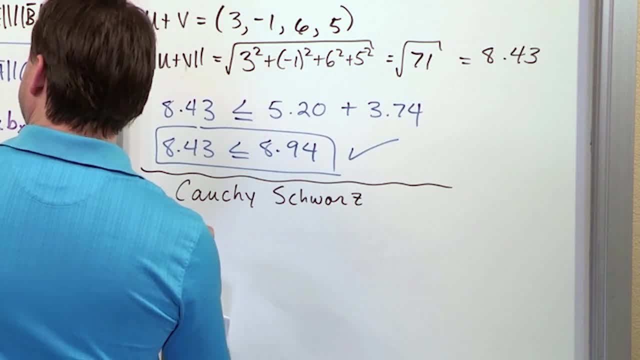 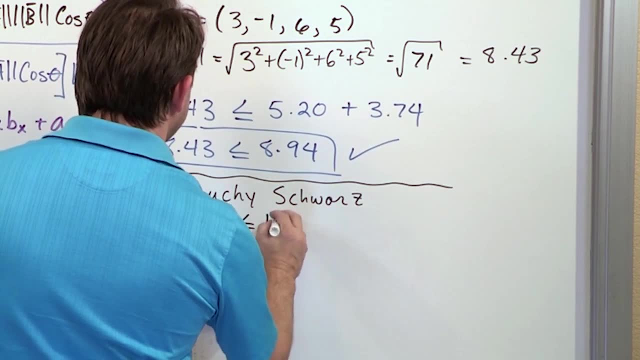 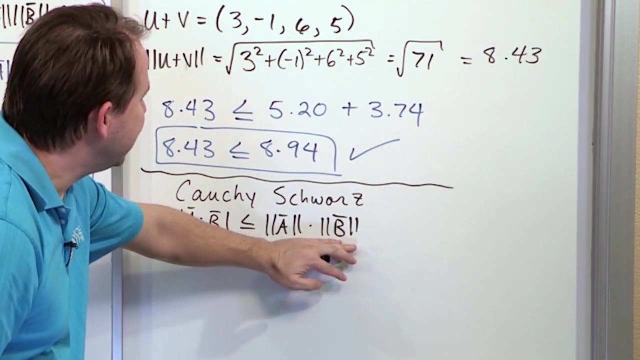 what was that again? We'll write it down. It basically is telling us that magnitude of ab, less than or equal to vector a magnitude multiplied by vector b magnitude, It should get something less than or equal to the individual magnitudes multiplied together. 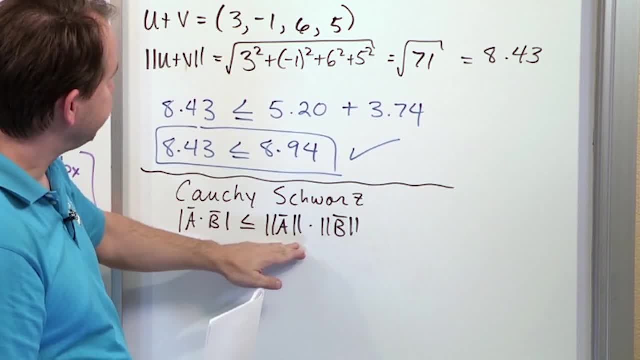 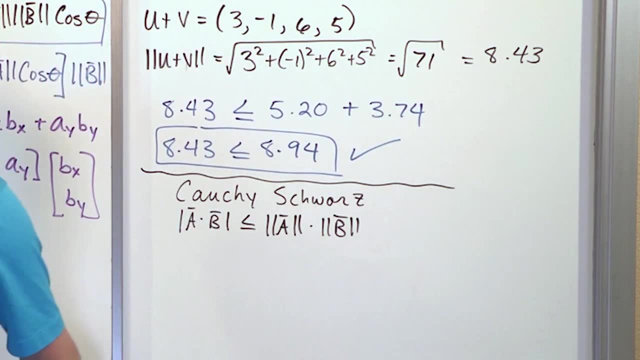 Now we already know what the magnitude of a is. We're using the same vectors here. That was calculated up there. We already know what the magnitude of b is, So what we need to do to get the left-hand side is find the dot product. 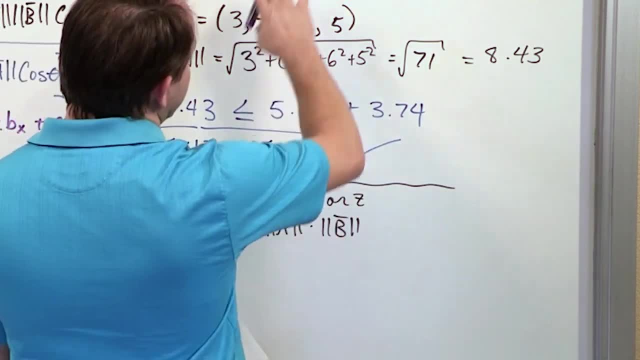 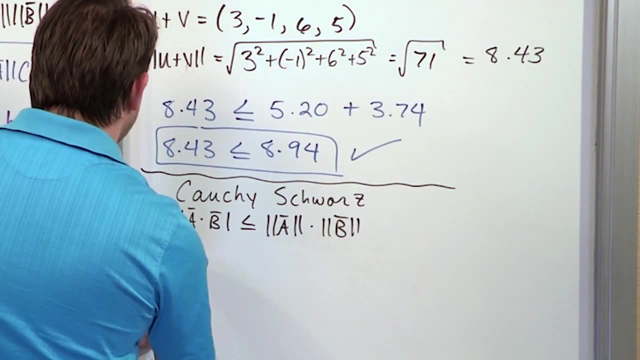 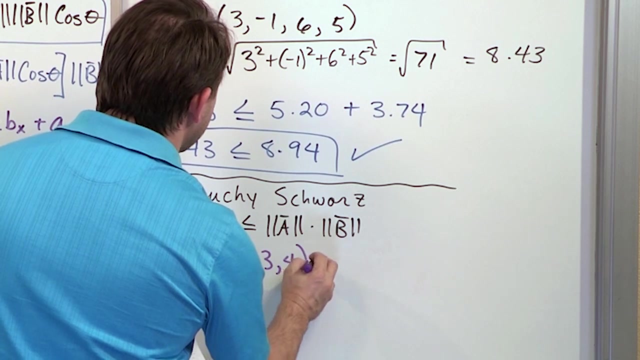 And we know how to find the dot product because we know what the vectors are. So, in order to find, in this case it's u and v, So I'll say u dot v. The u vector, don't forget, was 1, negative 1, 3, 4.. I'll just rewrite it here And we'll dot it. 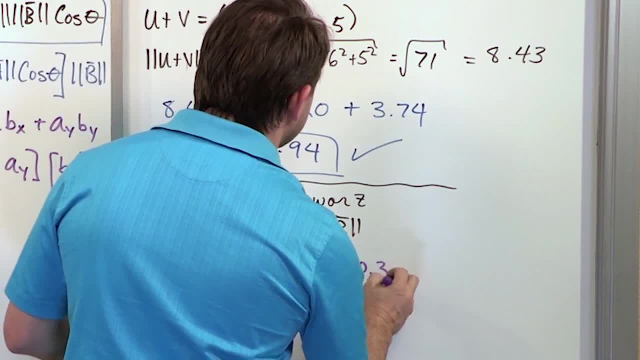 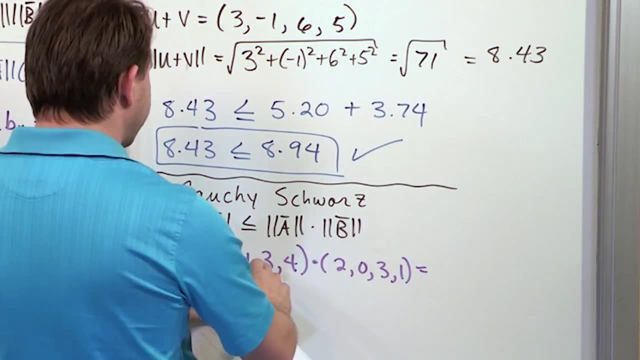 with the v vector: 2,, 0,, 3, and 1.. So whenever we dot these guys together, you look at the individual components: 1 times 2 is 2.. And then you have negative 1 times 0,, so you have 0.. 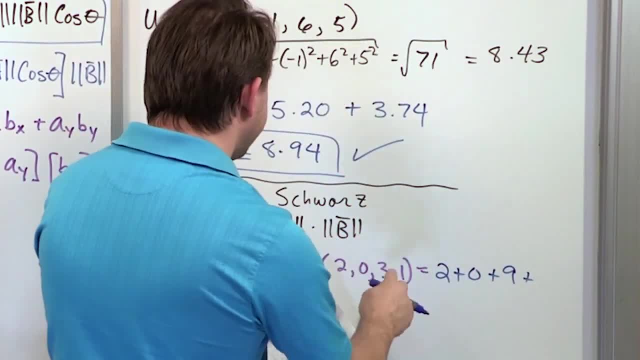 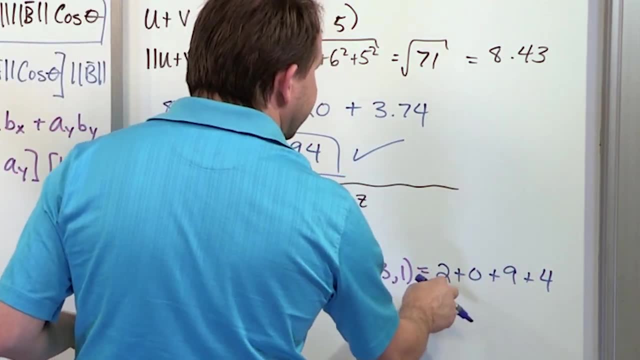 And then you have 3 times 3,, which is 9.. And then you have 4 times 1,, which is 4.. So u dot v B. this is 9,, 10,, 11,, 12,, 13,, 14,, 15,, so we have 15,. so we have 15 there. 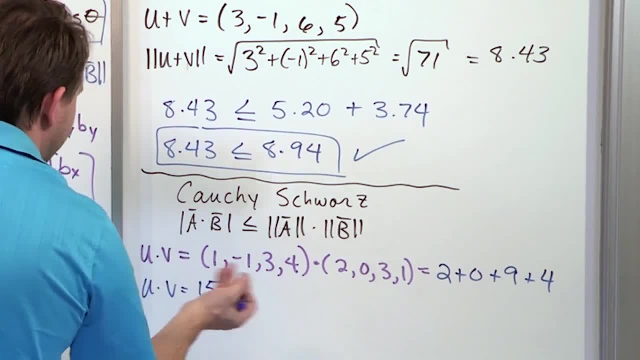 And, of course, if you take the absolute value of this, which is what we're doing here, the absolute value of a positive number is just a positive number. So to verify that it's true, the dot product of the two vectors when you take their absolute, 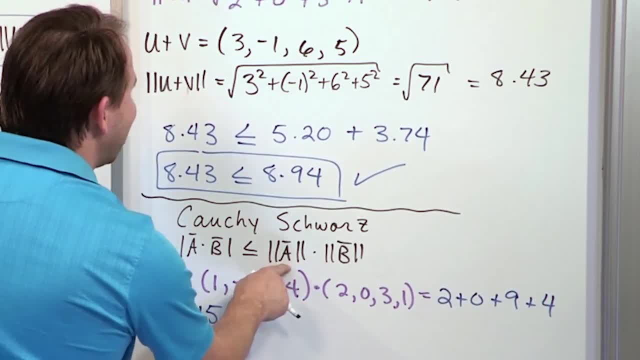 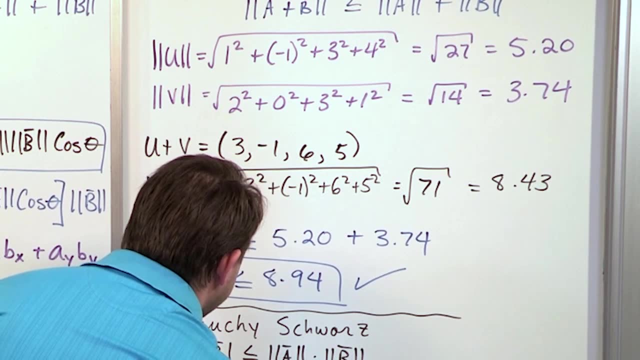 value is 15, and we're claiming that it should be less than or equal to the magnitude of a. magnitude of a, which is magnitude of u, is 5.20 times magnitude of b of the other vector, which is 3.74.. 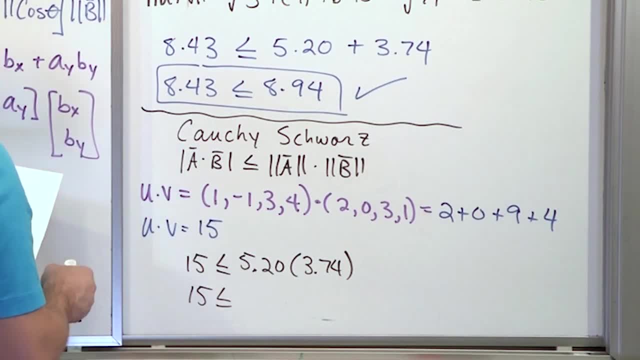 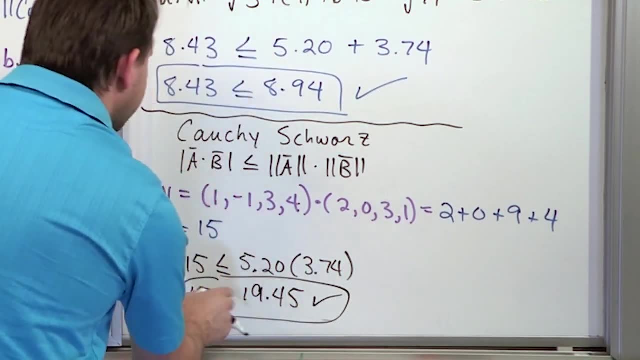 So what we're claiming is: 15 is less than or equal to. when you take 5.20 times 3.74, you get 19.45.. So it's verified: The number on the left is less than the number on the right. 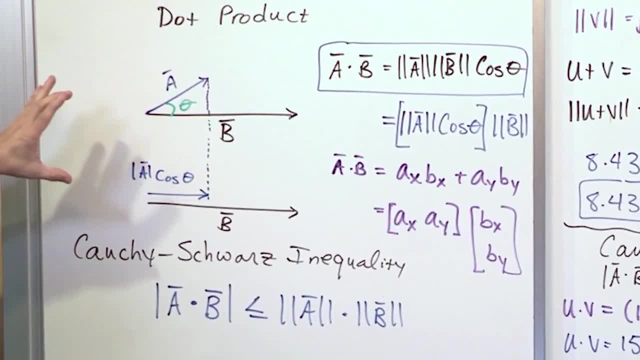 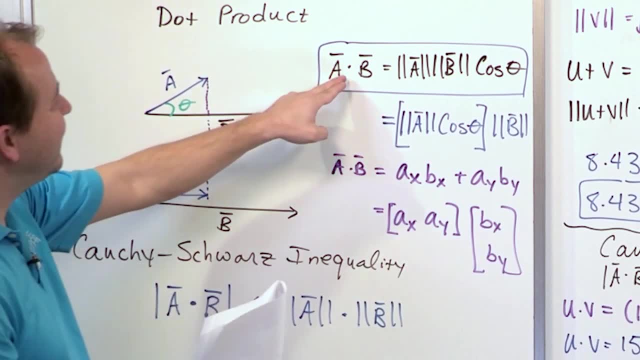 And again it all comes back from Cauchy-Schwarz with the definition of the dot product. Like when you have two vectors that are basically skewed relative to one another by an angle, then the dot product definition of it is taking the a vector, chopping it, finding its component. 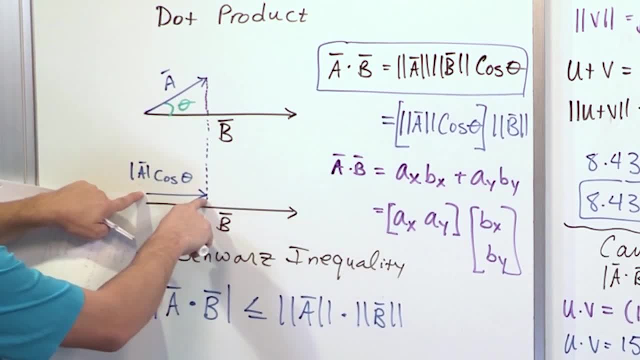 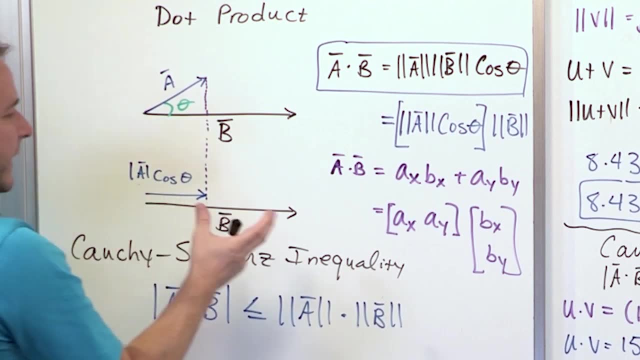 that lies along b. This component that we have chopped is always going to be smaller than the original vector a, because that's the definition of what a projection is there. So the inequality therefore makes a little bit more sense Whenever we take the length of this and multiply by the length of this, which is what's on. 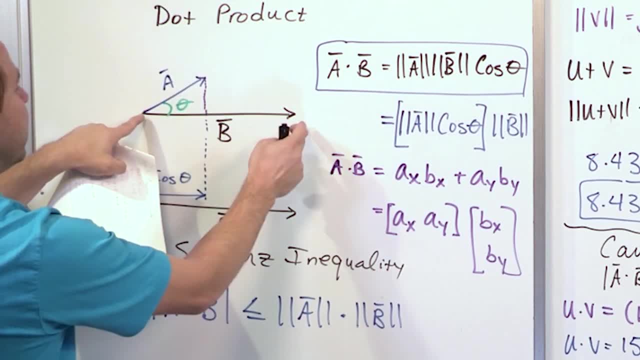 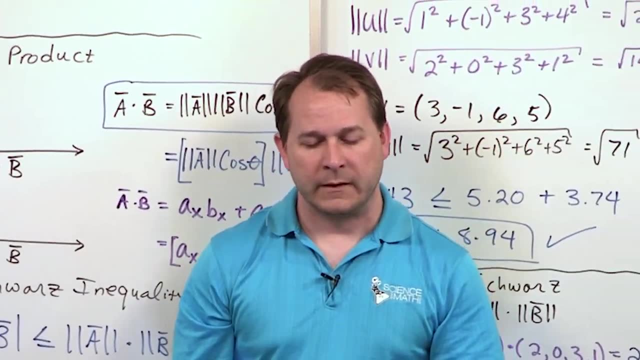 the left-hand side, It should be less than or equal to the magnitude of a, Less than taking the length of this vector times this one, because the vector a is going to be bigger than this projection. That's where that basically comes from and we're proving that it's true there. 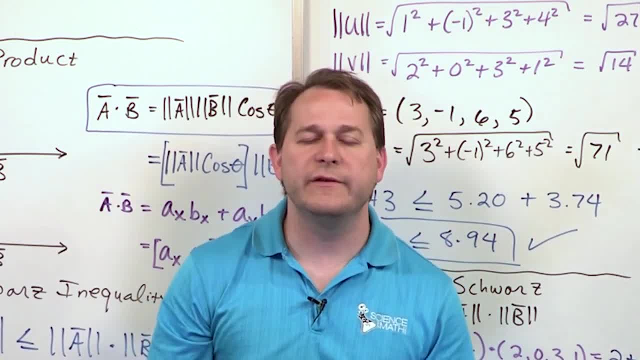 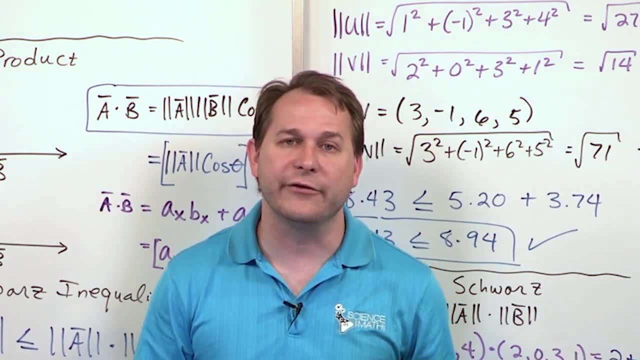 Again, when are you going to use these? You know we'll use them when we get into higher order vector spaces. We'll kind of use them as analogies when we go and transport ourselves into vector spaces later on down the road. But the short answer here is that in almost every linear algebra course you're going. 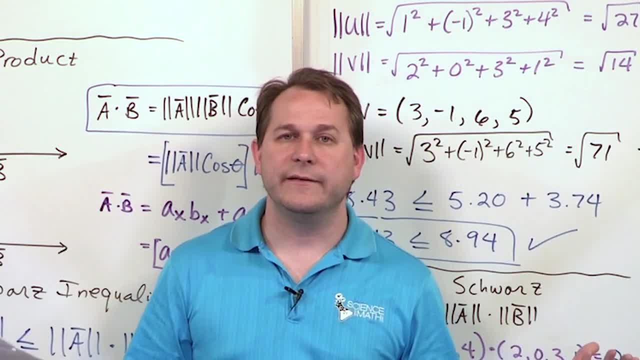 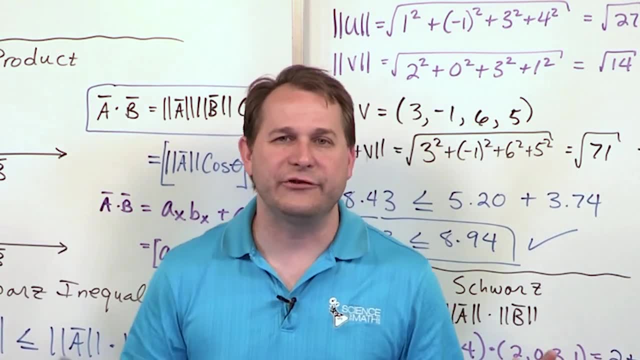 to start studying matrices and vectors right at the beginning, and then you'll have these inequalities here: the triangle inequality, Cauchy-Schwarz inequality, where you'll be basically asked to flex your muscles in terms of understanding vector addition and dot products. 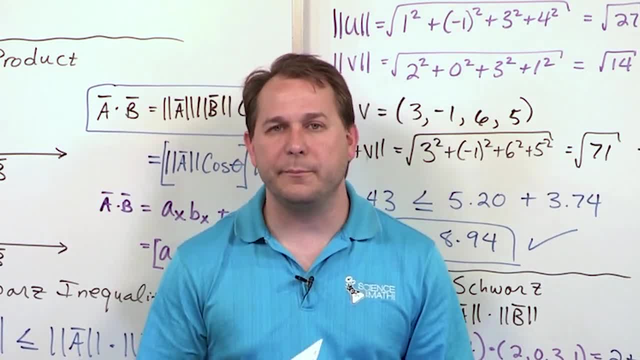 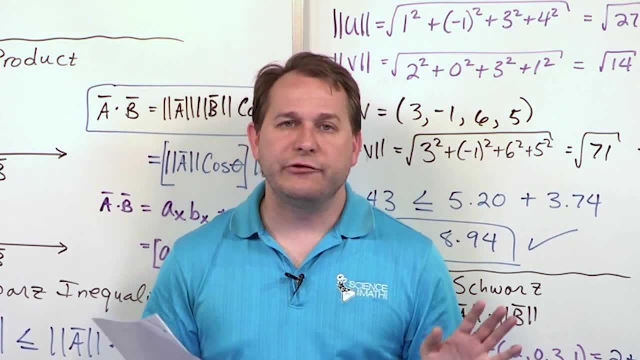 And so we're mixing vectors and matrices and such, and I think I've said enough times that they're basically belong in this class, because vectors can be treated as a matrix, as a column matrix, like that. So make sure you understand these guys. 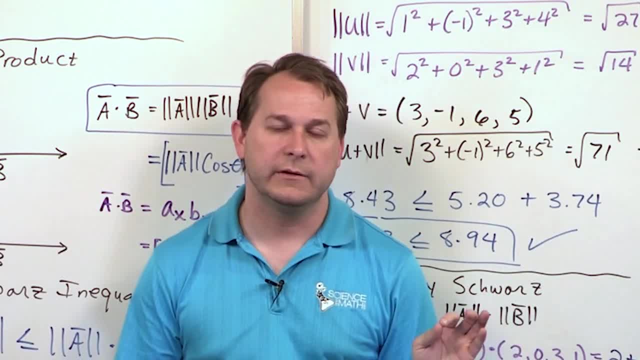 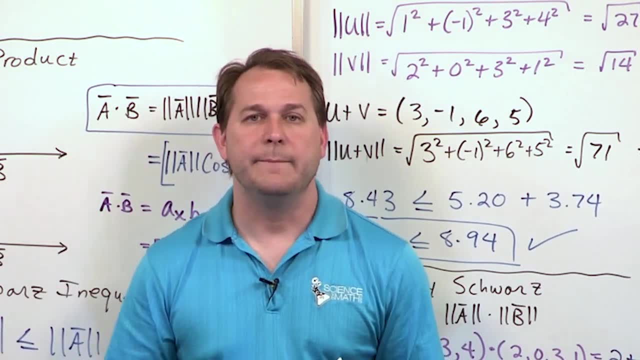 Make sure you understand how to verify some of these inequalities. Very common test question. And then follow me on to the next lesson. We're going to continue learning about vectors. Eventually we're going to get into matrix, solving systems of equations with matrices. 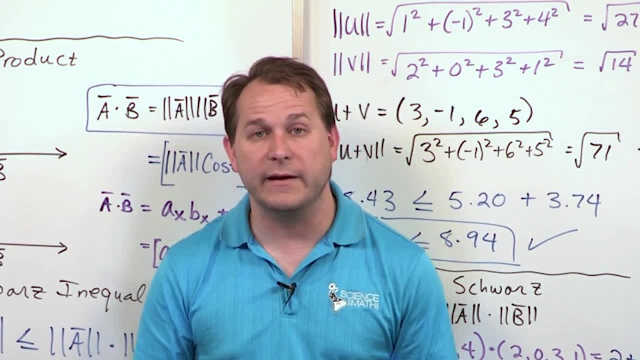 and inverses and things of that nature, and we'll just kind of go down the line, working everything with step-by-step examples. Learn anything at mathandsciencecom. 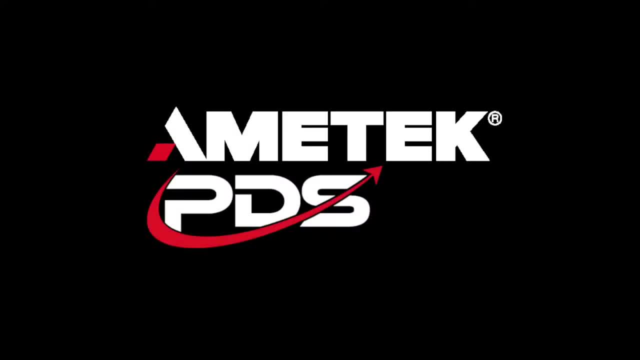 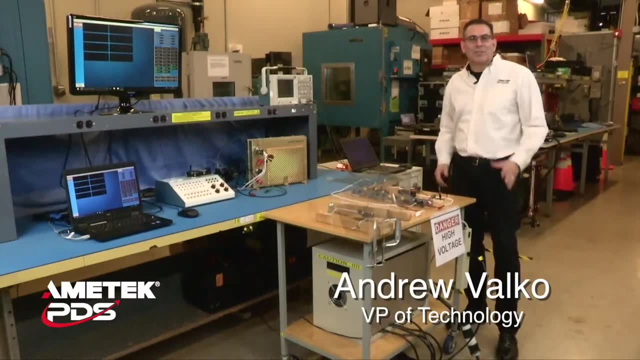 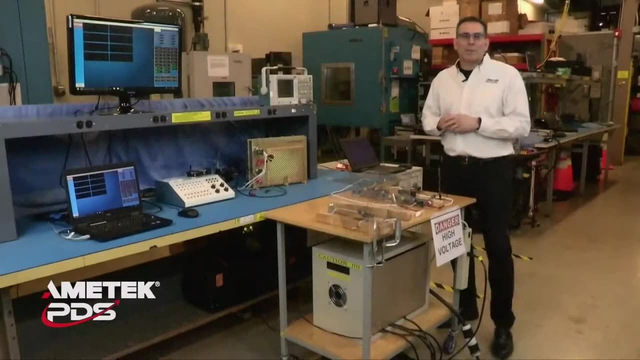 Hi, Andrew Velko here and welcome to the Power Labs of Ametek PDS. If you know anything about our business, we specialize in aerospace-grade solid-state power control, and that includes wire protection. One of the big and key advantages of solid-state is the switching speed and 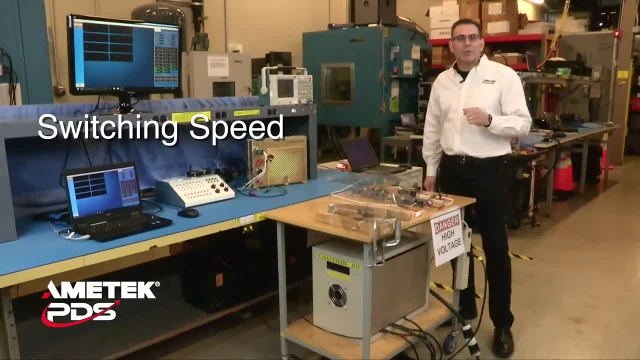 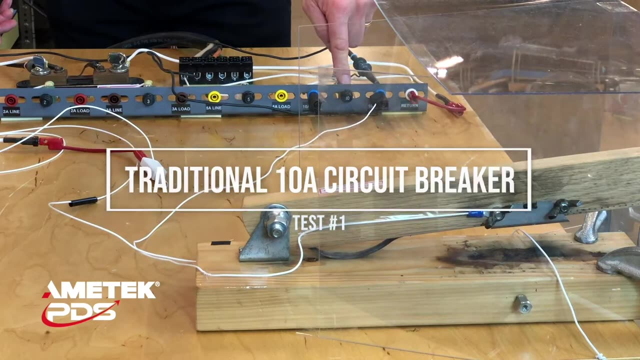 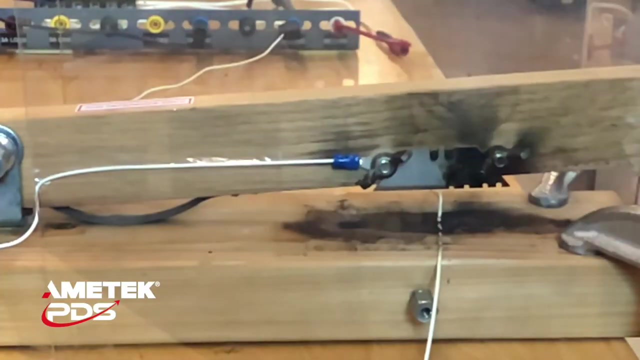 the ability to quickly interrupt a wire fault. Today we're going to do a quick demonstration that shows the speed advantages of solid-state technology and the benefits it provides in terms of minimizing collateral damage to both the wire bundle and the aircraft. Go ahead and work your way down the blade. That's pretty bad. Whoa, Whoa. Now you can. 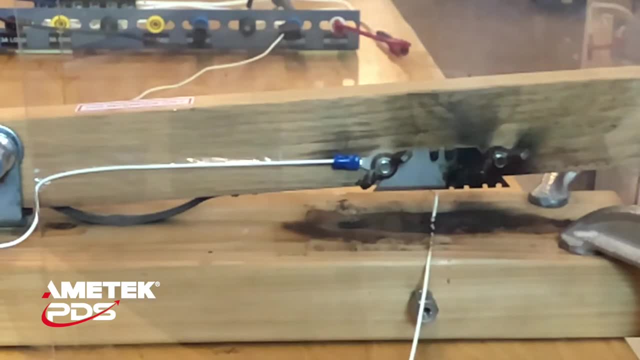 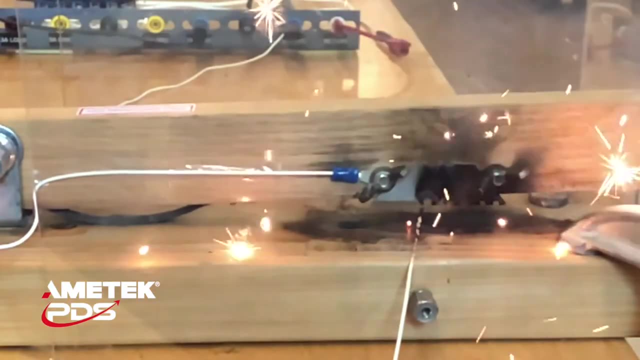 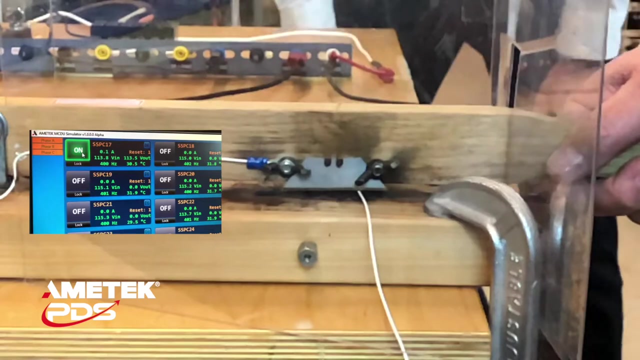 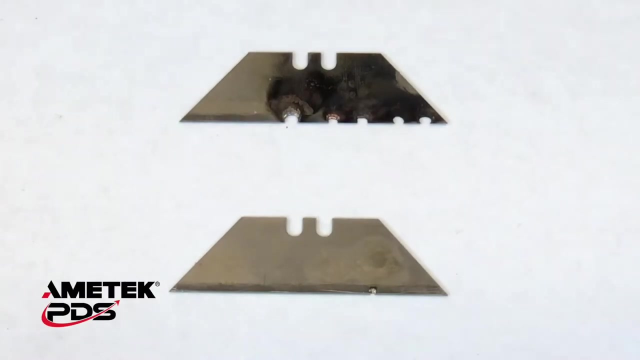 see he has to feed the wire through continually. Oh, we basically torched the blade. The circuit breaker tripped, The circuit breaker tripped, So it took about what Five of those until we got the actual thing to trip. Okay, so we've pulled the razor blades out and you can see this top blade here, This. 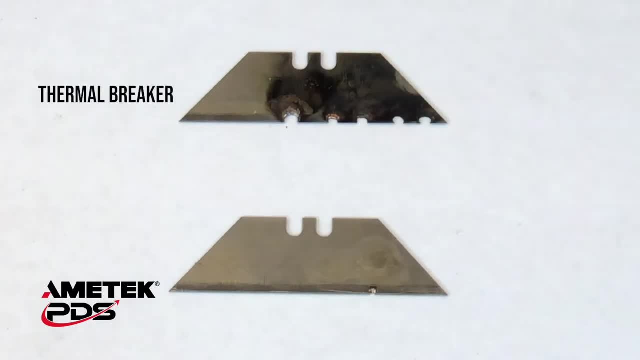 is the thermal breaker. You can see the five different hits, how it vaporized, basically the edge of the blade. And here is the one shot on the ACS PDU. You can notice a dramatic difference in terms of the amount of damage done to the blade and the fact that the SSPC. 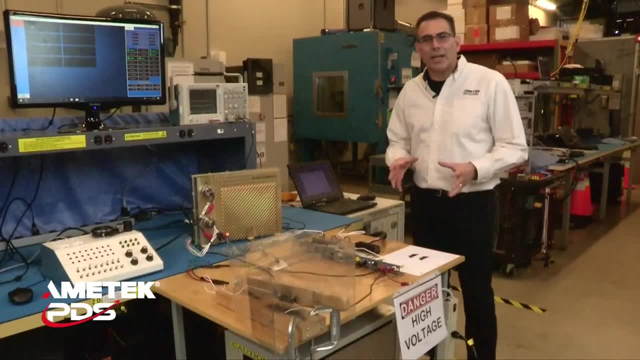 tripped the first time. So this demonstration gives a really good contrast between a thermal mechanical breaker and a solid-state power controller that relies on a shunt to measure current. You can see there's significantly less damage when a solid-state power controller is measuring current in microsecond. 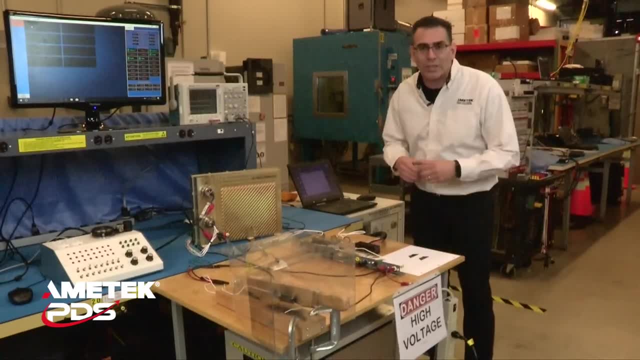 intervals and is able to basically interrupt the fault before significant damage is done. The disc is an ACS PDU. It's not going to be that much more, but it has to be very much more than the current score. Okay, a couple more.